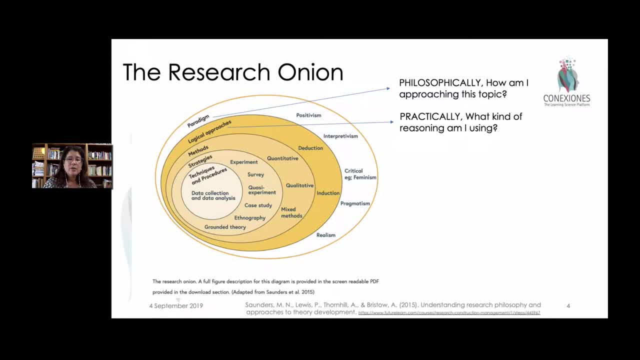 really dig deep enough and to think about this, but it is very important because we will talk about how some of the research findings that we look for are biased by our own belief systems. At the next level, though a little bit more inwards, are things that we call methods. 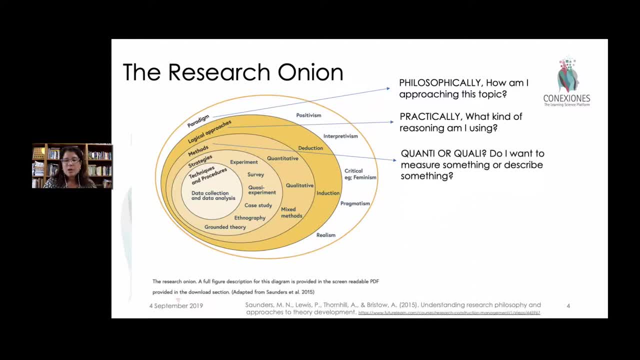 And this is asking us to determine if we're going to be approaching the problem through a quantitative or a qualitative or a mixed method structure. Okay, so do I want to measure something or do I want to describe something? So, basically, coming to that decision, before you launch into the research and collect data. 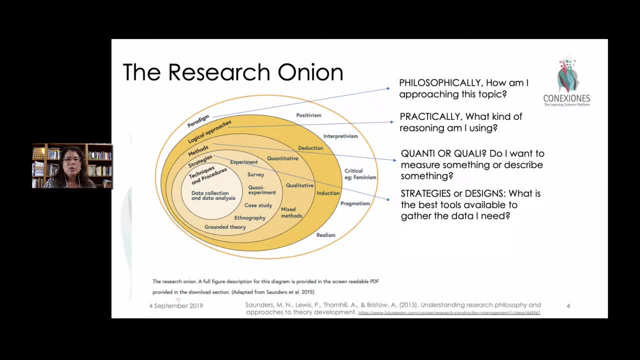 So, in order to collect data, you have to have a strategy or a design of how you're going to do that. And what's so interesting is these break down into basic tools. You know, am I going to use a survey or am I going to do an experiment? 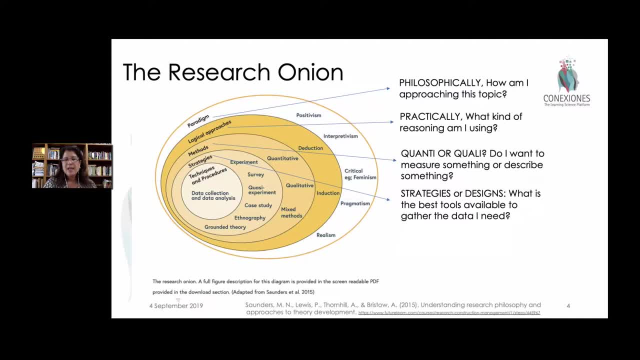 Shall I use a case study of an individual person. right, If you use something like grounded theory, it's because you're thinking of something nobody else has thought of before and you're coming up with something from the ground up. You're basically collecting a lot of information and saying how this points to something new that hasn't been thought of. 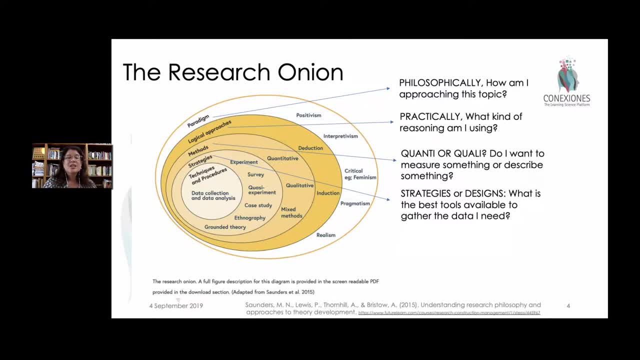 So these are strategies or research designs and then at the next level, we have the big job of data collection and we know this is a lot of errors that can occur as you collect data, and there's also a lot of errors that can occur when you analyze the data. 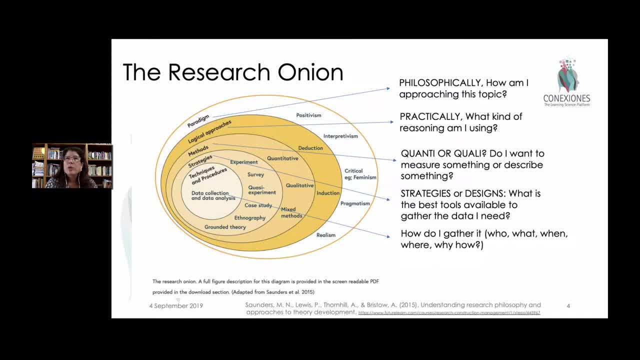 So when you collect it, you really have to think about you know who, what, when, where, why. how am I going to get the information? So if I'm going to do the surveys, how is it going to be distributed? How will I tabulate it right? 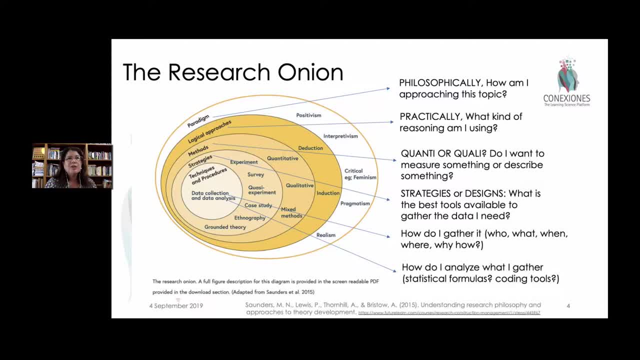 But then there's this next level of analyzing, Which is also very complicated. Once you've got that data and you've collected it, now, what are you going to do? Are you going to apply a formula to get a number, or are you going to you know? 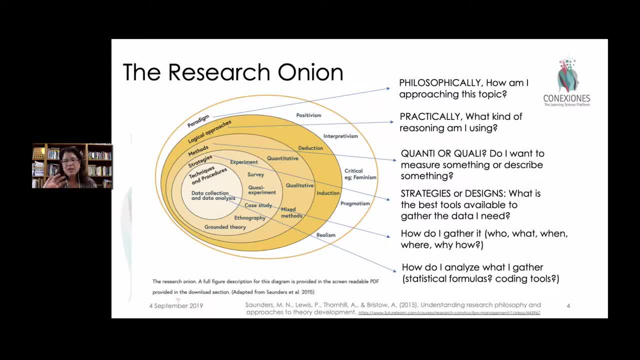 code, all the words that the kids said to each other to be able to, to categorize information? How will you approach the data collection and the data analysis? So these are the different layers of research that are indicated here. Now it's clear that something this is not a totally. even though it's complicated, it's not a complete. 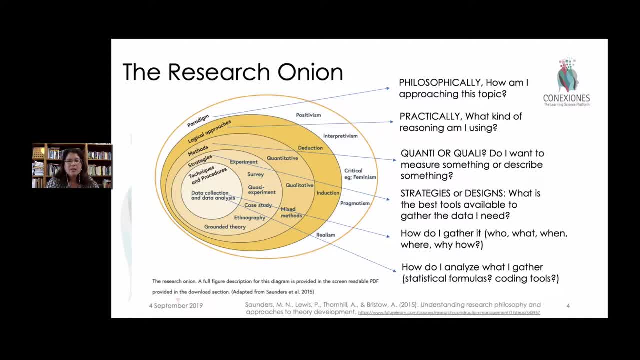 model because it is missing certain types of strategies or experimental designs. For example, another strategy or experimental design is looking at correlational studies, right, How two things might happen at the same time. Or looking at narrative studies, which are basically great descriptions of structures or contexts, or how classrooms might look, or whatever, right? 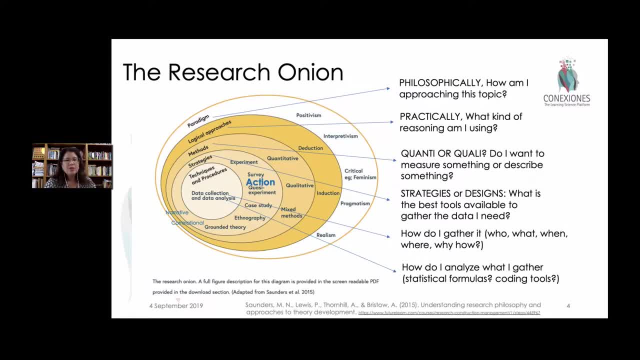 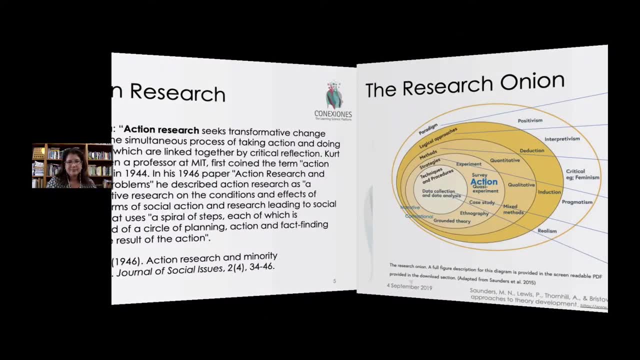 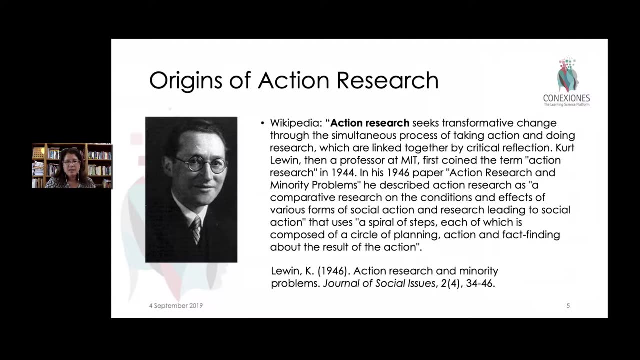 But then there's also action research, And action research is a different kind of design- research design that we're going to be focusing on today. Kurt Lewin, who was a professor at MIT, coined this phrase when he was looking at a specific problem within the MIT context. 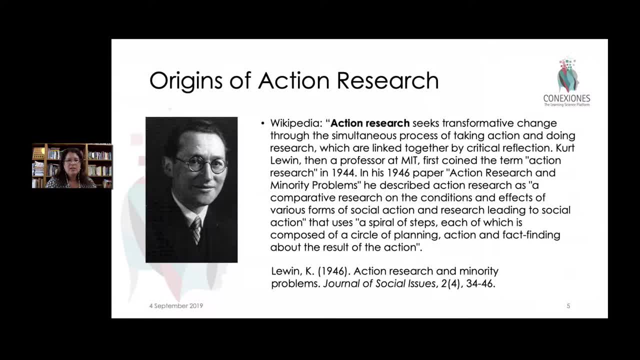 which had to do with looking at minority problems within the MIT structure. So he described action research as being a comparative research on the conditions and effects of various forms of social action and research leading to social action. So or change right. So basically, how does something occur within a social context that we take actions upon, or that actors act upon, and that change that other thing? 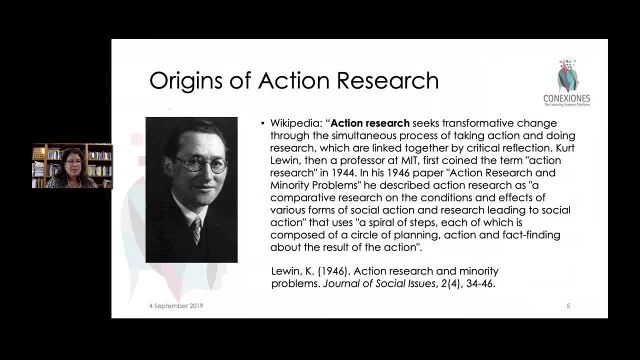 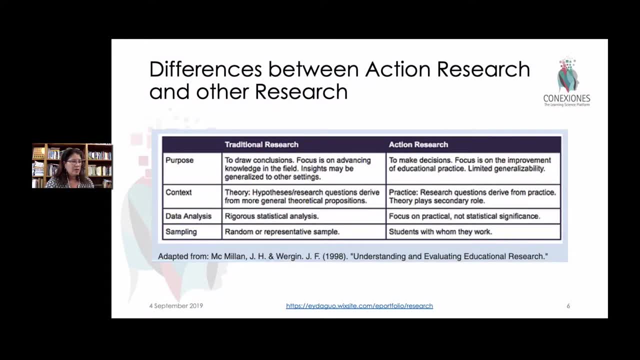 Okay, so that was the first time back in 1940s and that was something that over the past almost 80 years has really evolved into really getting into very defined areas, And so the biggest clear definition we have is that traditional research is trying to reach a conclusion. 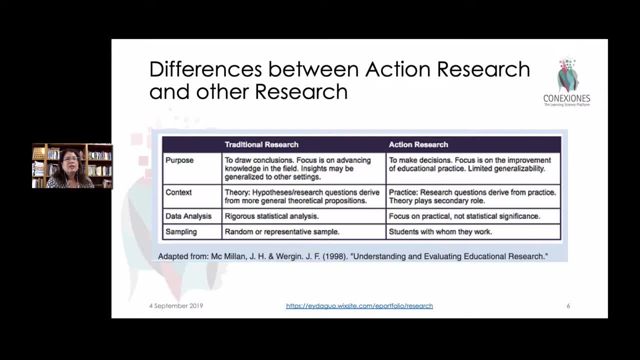 It's trying to give us a unique understanding. It's trying to give us a unique understanding A yes or a no on. is my hypothesis correct, right or incorrect? Whereas action research is conducted mainly to help you make decisions, Basically it's to resolve problems as opposed to draw a conclusion about something. 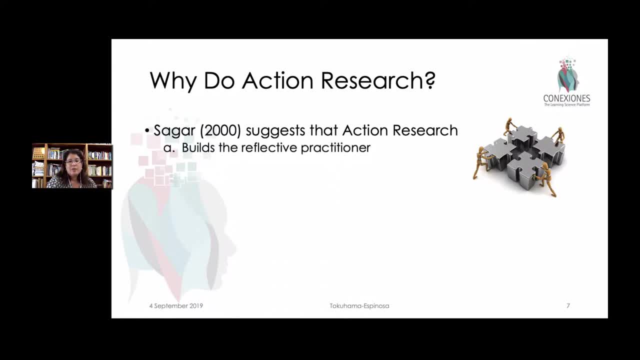 And many people are motivated to do action research for various reasons. right, Some people believe that it is the way to develop a reflective practitioner. This is why we have a lot of new models these days called the TGP. This is why we have a lot of new models these days called the TGP. 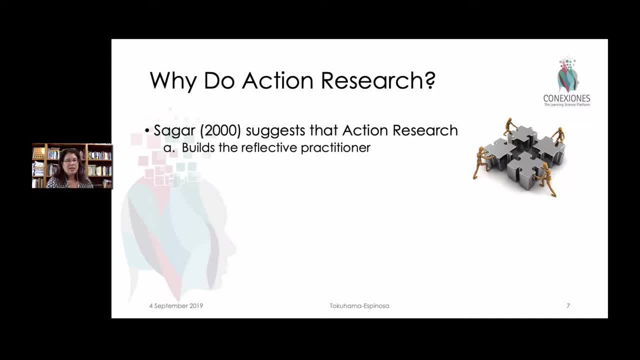 This is why we have a lot of new models. these days called the TGP, It's the researcher-practitioner model, right? So the researcher, practitioner means the person who is a researcher, but they're actually the practitioner, the teacher in the classroom doing things. 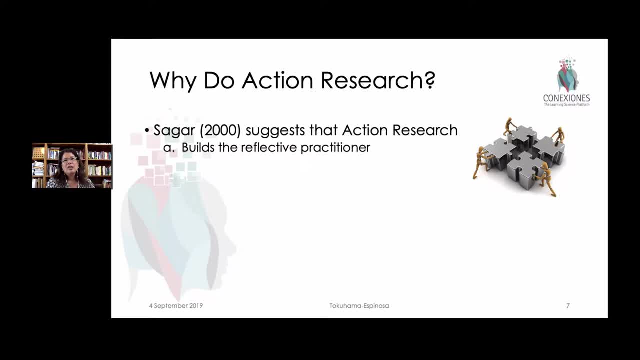 So the need to have reflective practice within that context. How do I stop at the end of every day and say, what did I do well, What did I do wrong, What can I do better tomorrow, in order to improve, continually improve my practice? 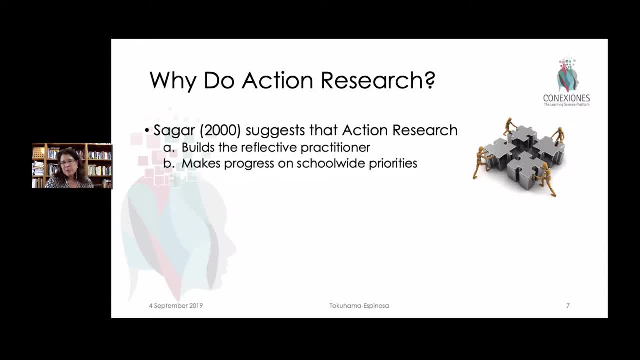 What can I do better tomorrow in order to improve- continually improve- my practice? Other people do action research because it helps promote school-wide priorities. Other people do action research because it helps promote school-wide priorities. school-wide priorities, For example, if we're all trying to reduce bullying or enhance social 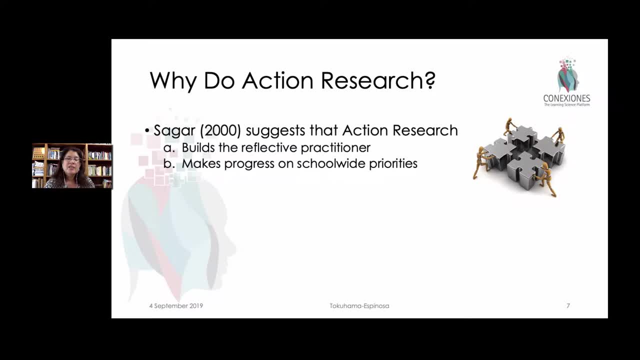 emotional awareness or get our test scores up, or something like that. different teachers might take on different types of initiatives to meet those shared goals, school-wide goals. It also, in some school contexts, builds professional cultures. In many schools, action, research is required of. 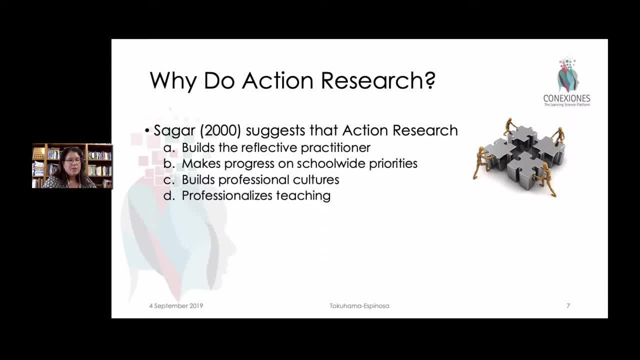 teachers every single year. This also professionalizes teachers. Instead of just saying, well, I had a gut feeling, I did this, you can say: well, actually, I did a research project last year that really confirmed this hunch I had about the way kids interact, or whatever, it is right So. 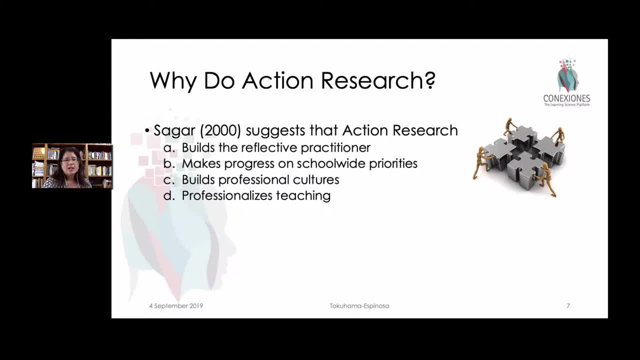 there's a professionalization element to this because of the documentation that's involved. We also think that it enhances the motivation and efficiency of people who might just be getting tired and worn down by their practice. It's very rejuvenating and interesting to follow up on. 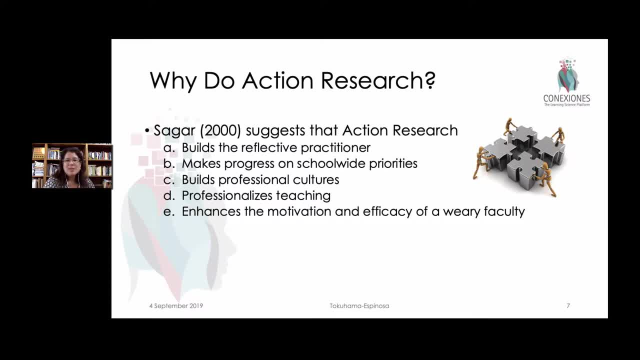 something like that That we're curious about. you know that pushes us to be students as well, right? So it's another way of energizing, maybe, people who've gotten tired of the same old, same old teaching routine. to have research in there really adds a new dimension to the job. Other people think it. 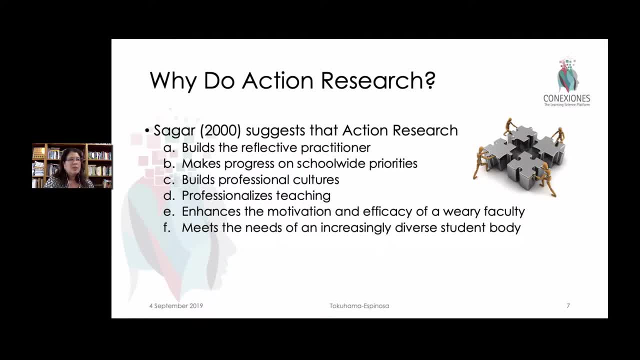 meets the needs of an increasing diverse student body because we're able to address multiple questions that can arise from different types of learners. And yet others think it achieves success by sort of aiming towards standard-based reforms. How can we have evidence in our pockets when we now approach? 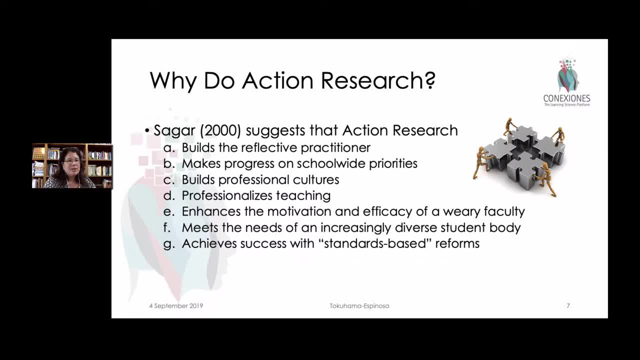 different types of policy decisions. So what I'd like to ask you to do is to think: you know, why are you doing the action research? That's a really important thing, to sort of own this process and decide- well you know, if I'm doing this for myself or for the group. So when we think about 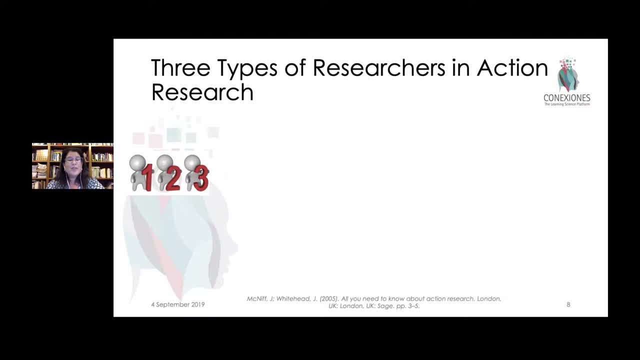 that there's basically three types of researchers. right, There are some people who are driven by their students. They're looking at their own agenda and they see that there's a need to do this, And there's a problem I'm addressing. There's also people who are out to change the world. Sometimes, 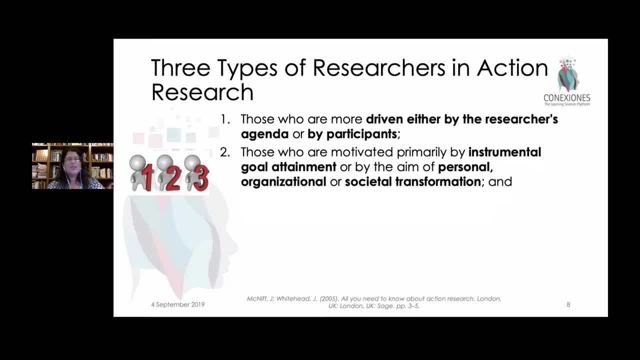 these are things as lofty as goals of you know. I'm going to transform society. I'm trying to create better people who are better society members and who care for each other. Or it might just be out for a type of instrumental goal attainment, like I need to score five points. 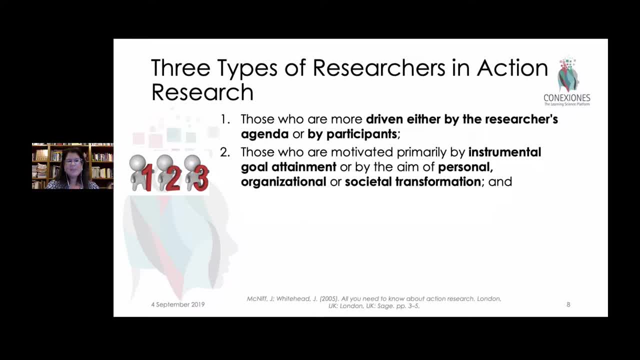 better on a specific standardized test or something like that right. A third way would be to look at this as a reflective process for personal change, or for changing, for example, the goals that we have as our department or a group that we're working within- right, But for personal change. So think about that, Decide which of these. 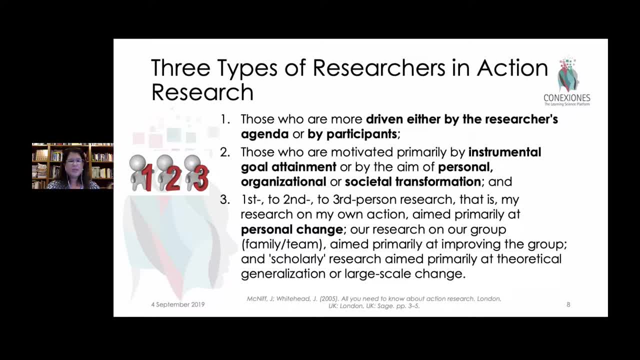 types of a researcher you are when you're doing action research. Are you driven by your students? Are you driven by this maybe greater goal- that's been probably something extrinsically imposed upon you- Or are you doing something very internal for personal change and growth? 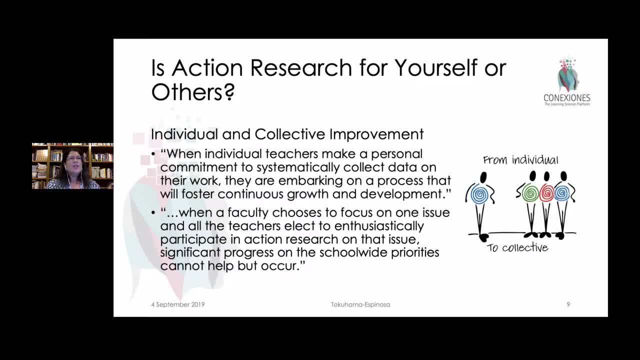 And, at the end of the day, what you're doing is you're doing something very internal for personal change and growth. And, at the end of the day, what you're doing is you're doing something very internal for personal change and growth, And what ends up happening is that you are doing both things right. You're doing things for yourself. 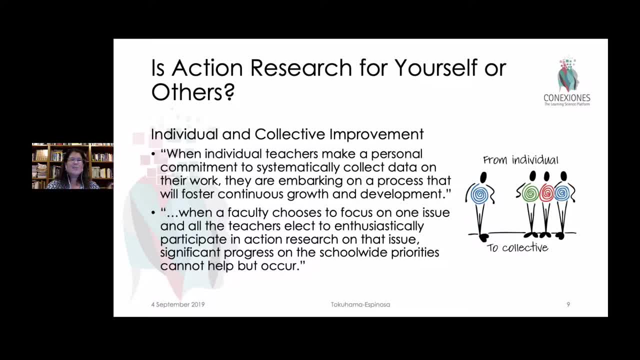 but also for the collective good. You are all taking on some research that may very well improve the chances that other teachers in the future can learn from the things that you've learned. So, while it's addressing a particular personal need that you've identified a problem, 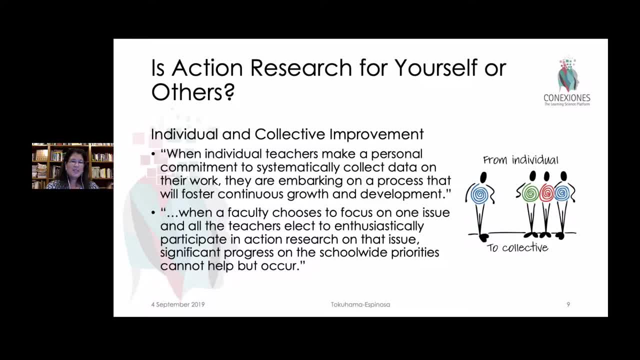 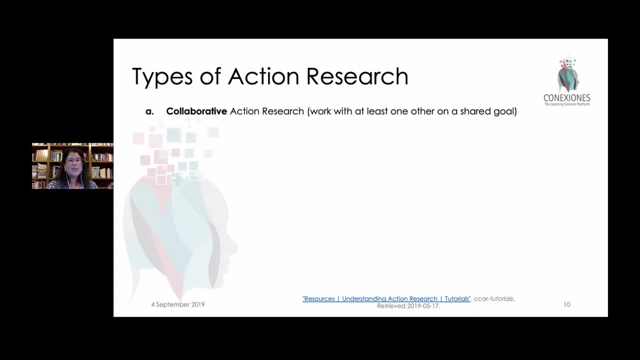 issue for you. it's also something that will largely benefit the community at the end of the day. So what are you doing? Are you doing collaborative action research? This means that you're working with at least one other person- maybe another teacher or TA- on a shared goal. 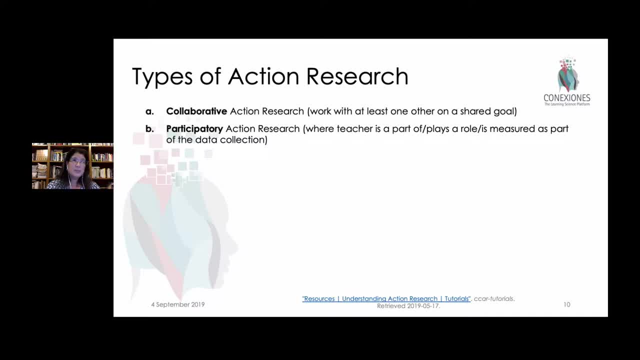 Are you doing participatory action research, which tends to be the most used within schools? It's where the teacher is actually part of the entire learning process and their actions are also measured as they're being done. So what are you doing? Are you doing collaborative action research? This is 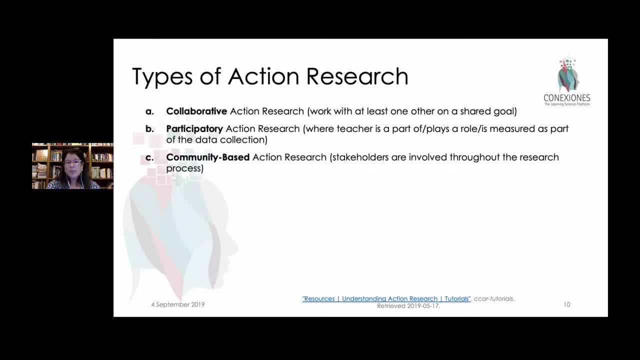 where they go through the process as well. Are you doing community-based action research? This is where different stakeholders from the community structure are also involved throughout this entire process. Are you doing youth action research? This is something where maybe your students have laid out a plan for you that they're going to do something, but you're going to be. 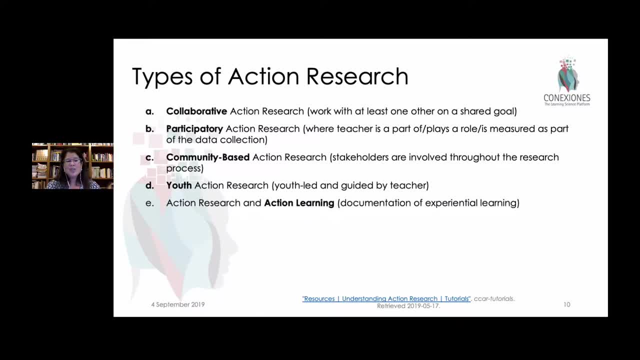 doing the documentation of all of this? Are you doing action research for action learning? This is if you were somebody going out to the fish pond and teaching fine, culture-based education, education. So what are you doing? Are you doing collaborative action research? This is where 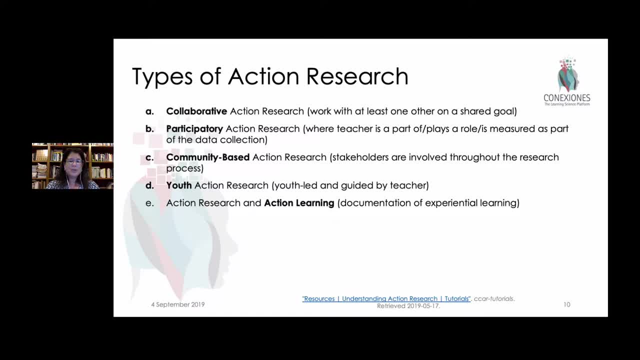 you're going to be based on contact with your local environment, for example. So, experiential learning: Are you doing something that's called PILAR right now, This participatory action, learning and action research, which really hovers around 21st century soft skills? right, Are you looking? 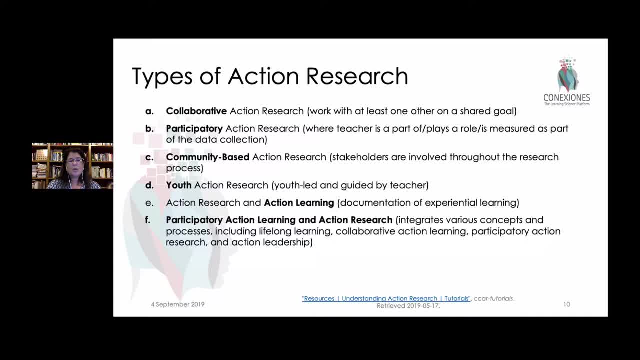 into lifelong learning or collaborative learning structures or ways to do leadership skills with students right, Or are you doing collective action research, where maybe your entire department has a single goal, but you're doing collaborative action research? This is where you're going to be based. 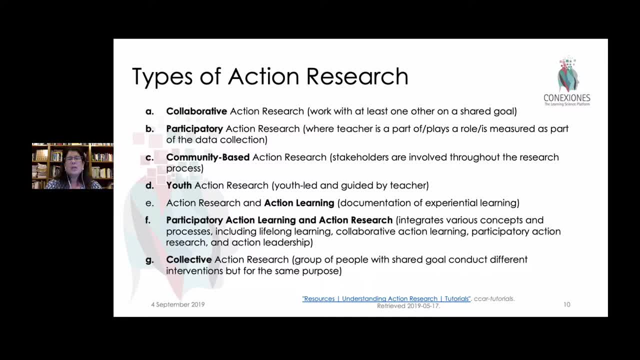 on a specific goal about doing things. For example, we want to enhance social-emotional learning or reduce rates of bullying or whatever. But different teachers will have different things, they do different types of interventions And then after a certain period of time, people get together. 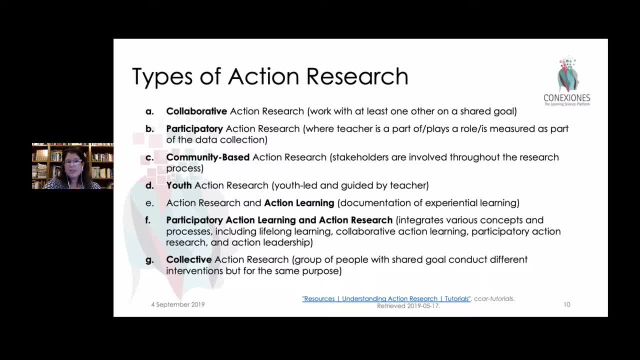 and they share the results of their collective efforts to reach that specific goal. Think about the type of action research that you're doing, because the more specific, the more precise you are with the type of research you're doing, the easier it is to choose the right kind of tool. 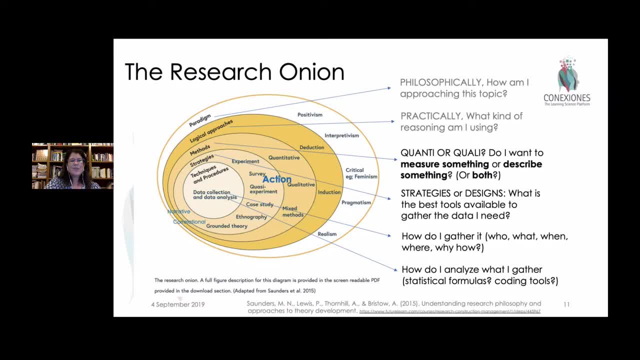 to gather the data and to measure things. So we go back to our onion again, okay, So in action research, we're going to not specifically address those first two layers of philosophically. how am I approaching this? Although at the end of the day, of course, this does come out and it is a 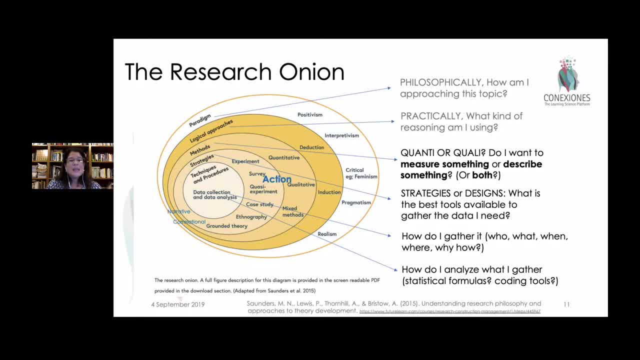 big part of the discussion. We haven't done this explicitly enough because this structure is also designed for things, like you know, five-year-long PhD thesis study things. So they're really really long-term things where you are able to take a lot of good time to reflect and think about. 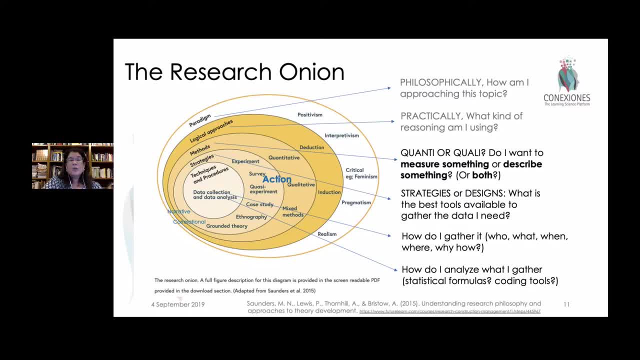 that philosophical approach, And also to decide and look at multiple ways of approaching. you know the reasoning that you're going to be using. What we will be asking you, though, is to decide now. are you going to be approaching this quantitatively or qualitatively, And are you going to use a? 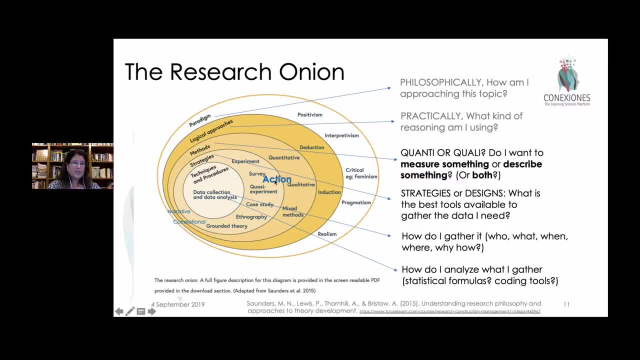 strategy or design. that is pretty much we're leaving. it's action research, but some of these can also be tools for action research. So we're going to talk a little bit about that in a moment. We're going to talk about that in just a second right, And then, when you think about how you're 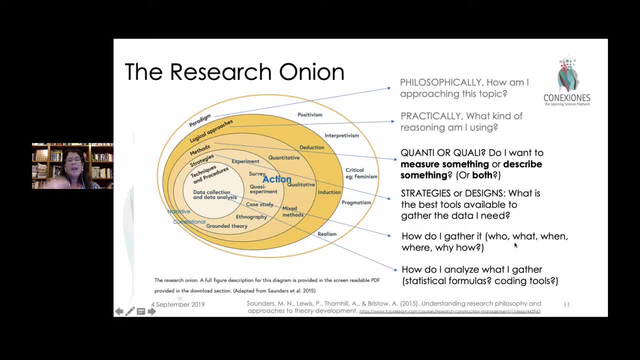 collecting the data. make sure you go through those processes really clearly and how we analyze that. We're going to look at those in the steps in just a second. okay, So globally, if we skip those first two steps, the very first thing we're asking you to do is think about: is this quantitative or 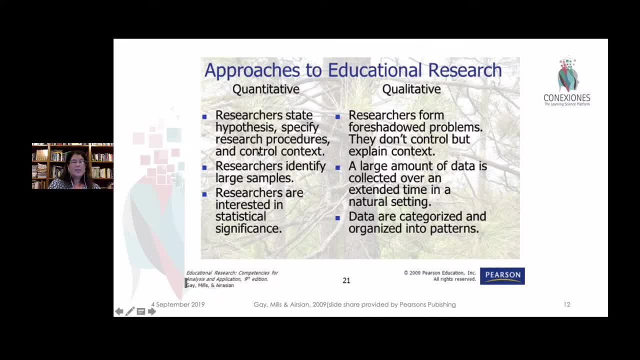 qualitative And a quantitative question is going to have a hypothesis and it's out to show X or Y is true or not right, Whereas qualitative is out to do a lot of problem-solving kind of things. It's anticipating answers but it's not out to 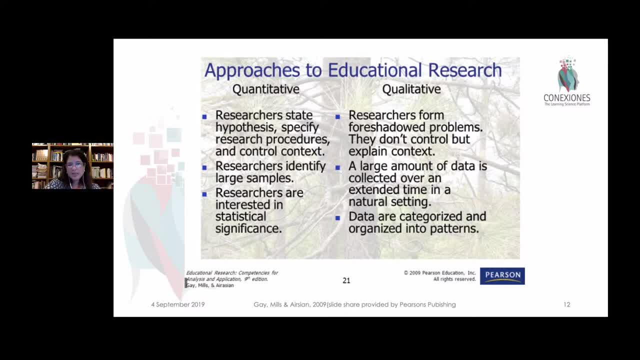 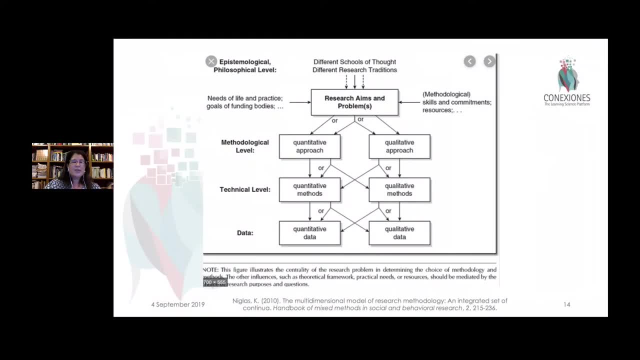 measure, but out to more or less to describe the actual process. So this means, in our very first step then, when we're looking at this idea, are we looking for quantitative or qualitative or mixed level data? This graph is is a pretty straightforward. look at this, you know it comes. 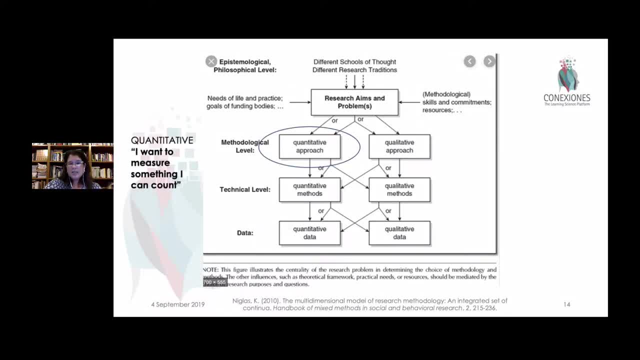 from Nicholas and the first level is okay. are we doing this quantitatively, You know, am I measuring something? I want to measure something I can count? Okay, Are we doing this qualitatively? I want to measure something I can describe, right, So think about that to yourself. What? 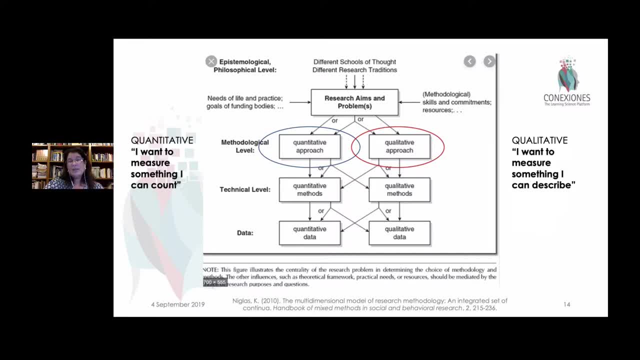 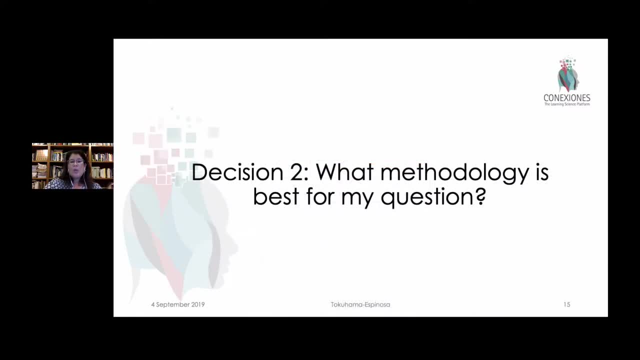 is it that you're out to do and make that first big decision? And if you say to yourself both, then that's called a mixed methodology, Okay. The second question then is what methodology is best for my question? Okay, So that means you have to look at the second step and decide at the 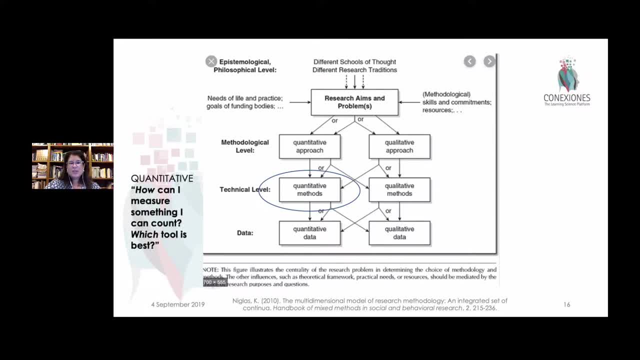 technical level. then how can I measure this? You know how am I going to gather the data. How can I measure this? Which tool is really the right? one Same thing with the qualitative right, Which of what I'm out to measure? So, if I think that I'm going to increase critical thinking skills, 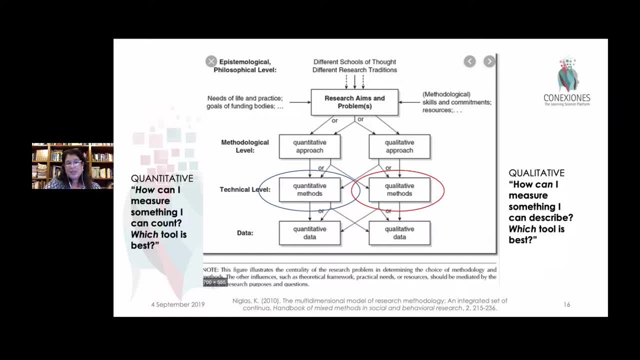 I should not use a multiple choice test to do that, because the tool is totally incompatible with what I'm trying to measure. Right, And we'll get to that in a second. And that has to do with them validity of the data that we're gathering, because when you say, something is measuring. 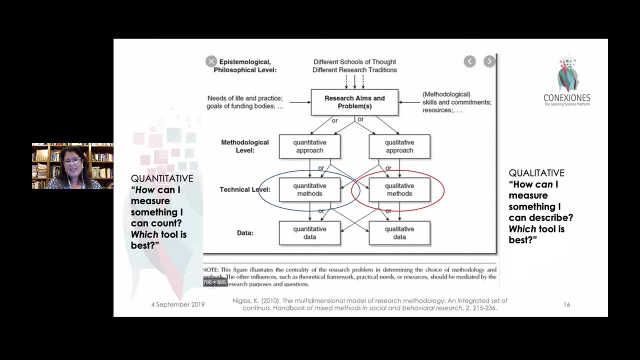 something and it's really not. that's not valid, Okay, So we'll talk about that in a second. but thinking out to yourself what kinds of tools exist is a questionnaire A good thing. Should I interview students? Should we have small groups work on things? Can I do a pre or post-test kind? 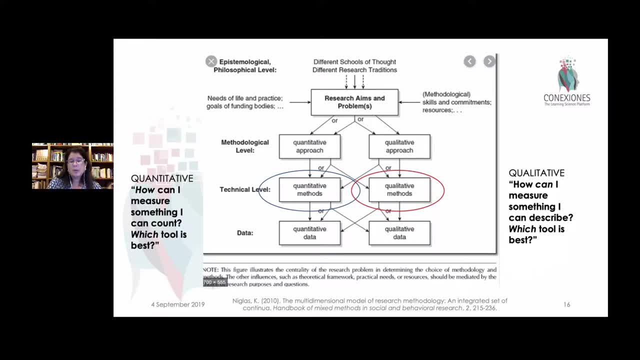 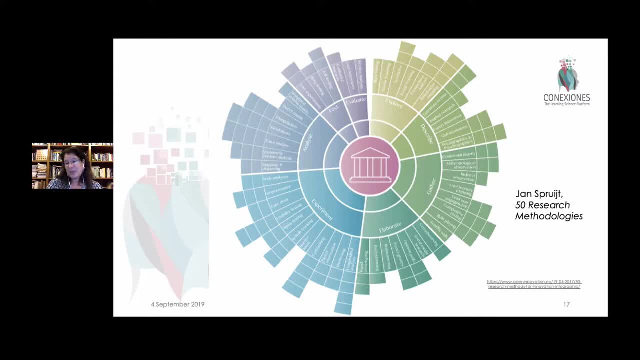 of a thing. Think about all the different tools that might exist that might be appropriate for your question When you get down to it- and I will be sharing this in class. I just think this is very pretty Okay, Jan Spruyt. she came up with this pretty cool idea of plotting out all these. 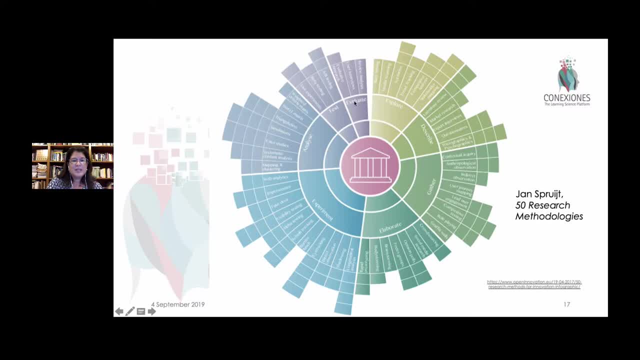 different types of tools. There's lots of different types of things that help us test or evaluate or explore or describe, And I'm going to talk a little bit more about that in just a second, And then you'll hear about Tracey at the end of the video. So, after you've analyzed and analyzed- 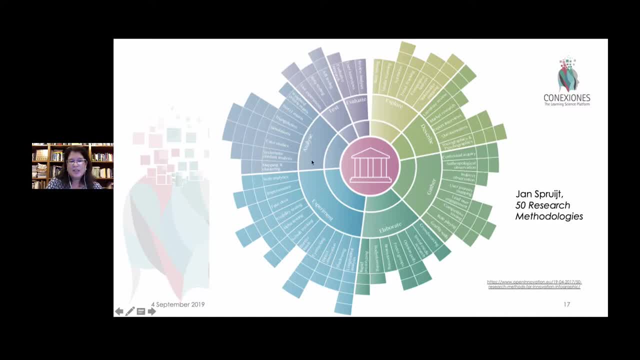 there's a lot of different sub elements here, like chce is sort of put on this beautiful, beautiful graphic here. This is not to scare you, It's just to sort of remind you. there are a whole lot of tools out there And the big idea to carry away from this is that. 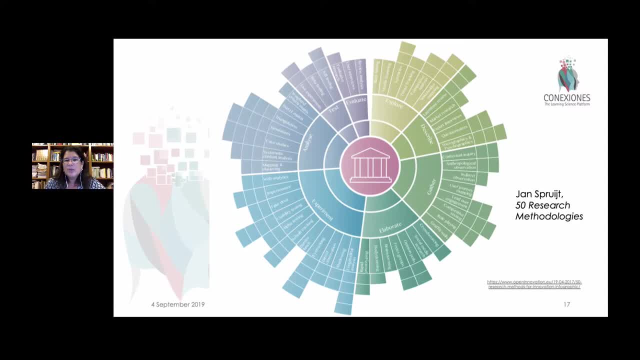 you can do action research with just about any one of these tools. Okay, The type of research, the fact that you're doing action research as opposed to an experimentation or other research. you have a very, very good chances of doing it, because it's interesting to know. 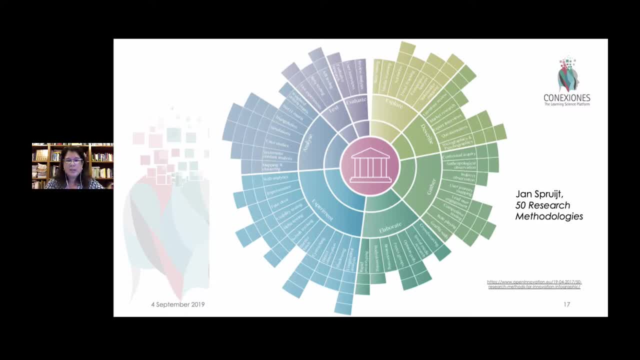 things like that doesn't exclude the tools, Okay. So just be clear on that. And we have done a lot of mixing and matching. She's called this 50 research methodologies. I would actually call this outer circle tools. These are different ways of doing things. right. You can have 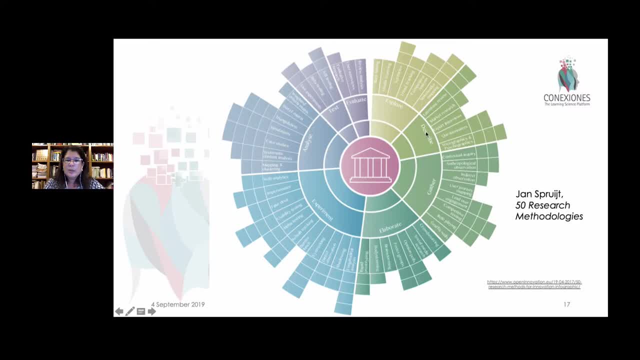 case studies or you can use systematic literature review. You can observe people doing brainstorming or you can have role-playing. All of these things, to me, are the activities. Those are tools you can use to gather data, but it's just best to know that, as you're doing action research, you're not 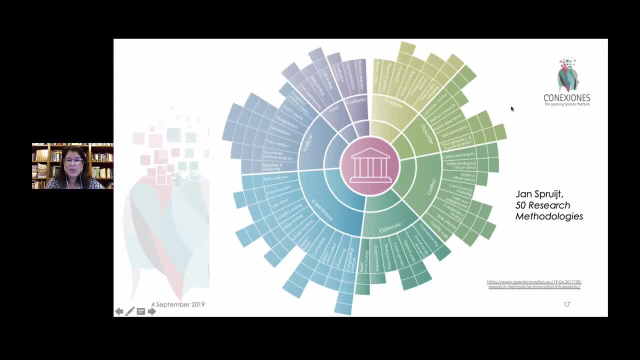 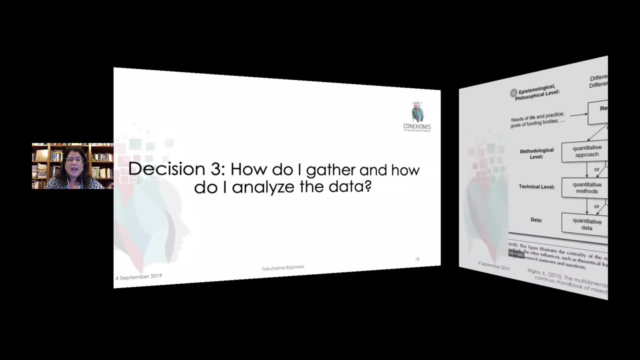 excluded from any of these interesting tools. You can use questionnaires or interviews, and you can use other types of experimentation. All of that can be within action research. Okay, So then the third level question is really: how do I gather this data and how to I analyze it? 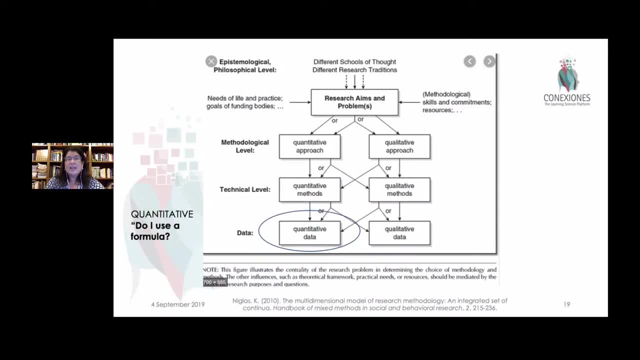 right. So if you're doing the quantitative data, at the end of the day you may just be asking yourself: okay, what's my formula? So am I just subtracting pre-test scores from post-test scores or just find a difference, or you know what am I trying to do here? And if it's qualitative, 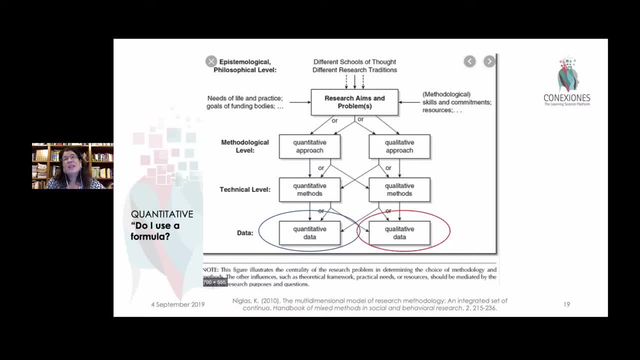 data. believe it or not, the analysis of qualitative data is really really probably a lot more time consuming than a quantitative data, because you may have to do things like coding. I'm listening to the dialogue of the students and seeing how they interact And I've got my own notes and 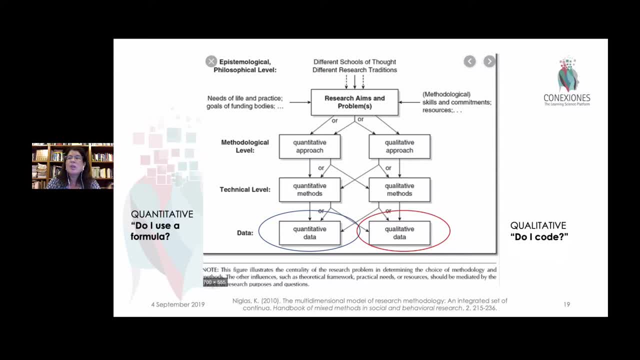 interpretation, but I've also coded for the numbers. So I've got my own notes and interpretation the number of times that they've used specific key emotional vocabulary words or something like that. right, So the coding you can use. actually quantitative structures within a qualitative. 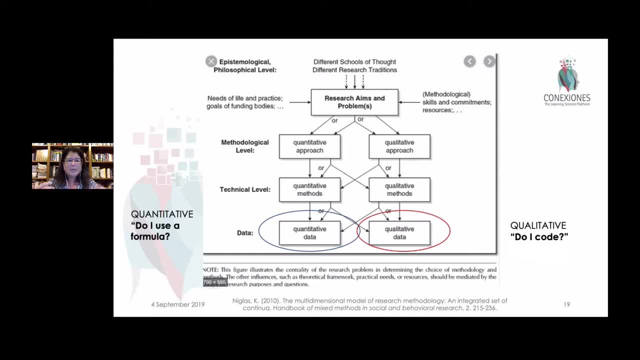 analysis. So that's another complicated thing to think about. but just the idea is: how will I gather the data and what would be the most appropriate tool, And then understanding that the process of analysis is one step further. It's not just that I have all this cool data. 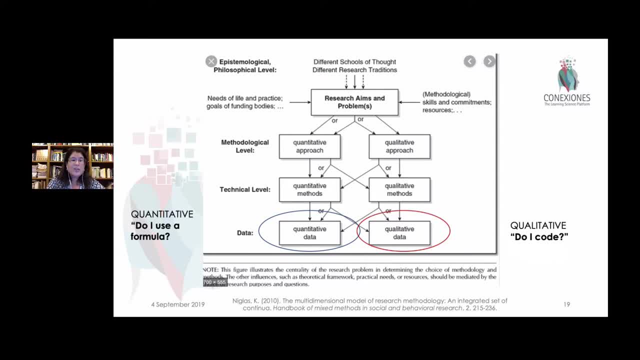 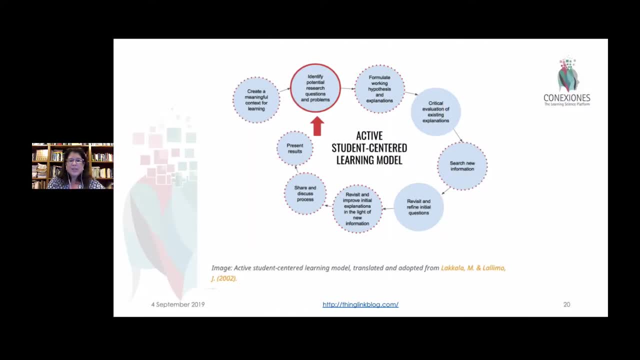 Now, how do I actually analyze it? We'll be based on another step. It's either a formula tool, it's looking at coding or something like that. So now let's look at a bunch of models about action research. This is a very student-centered model. I'm thinking about my kids I've created. 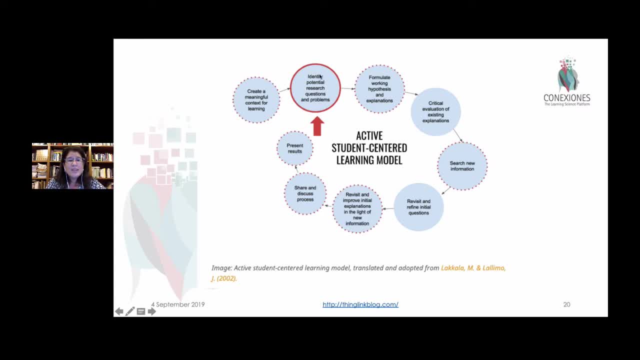 this great classroom, but I see that there may be some problems going on there still that I want to fix right. So I have this hypothesis that some of these kids are grouping together and there's this negative clicks forming and they're starting to bully each other, And so I'm going to look at 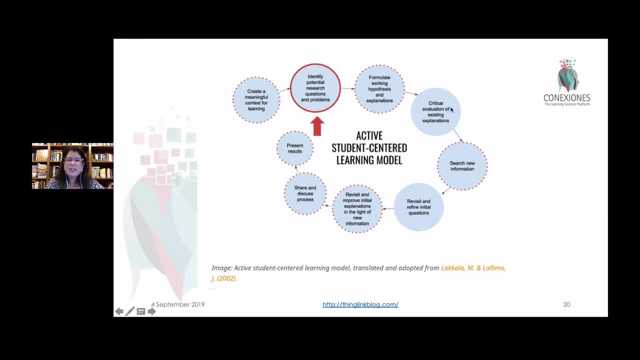 the literature on this and the fourth grade kids sometimes do that, And I'll look at all the things and I'll come up with maybe a different kind of a hypothesis based on all of this new information. And all of that may just very well change my question. Remember, in the prior class we talked 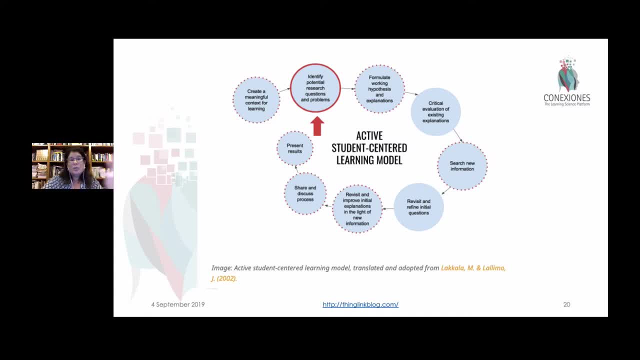 about radical neural constructivism. It's the way that we interact with our world has changed. each time, Even if we're having the same experience, we're actually interpreting it different because we already have that experience once before. right, So the more ways we take in information, 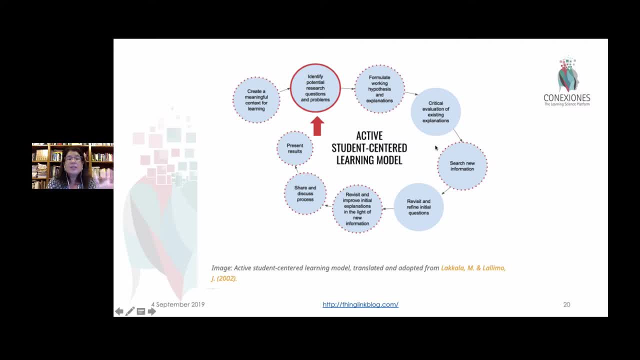 now we're going to look at our research question differently because we've had a lot of different literature on this. So we're going to look at our research question differently because we've had a literature. So this is what's going to happen during your literature review: You're going to 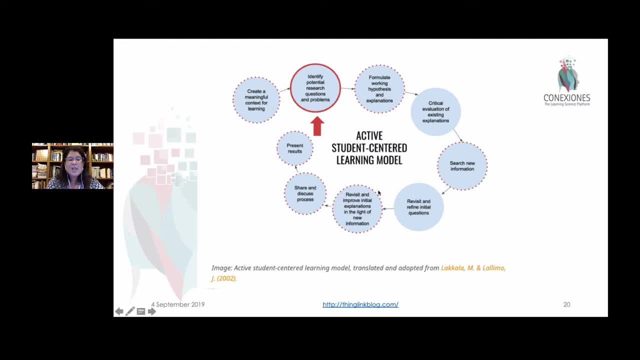 begin to rethink your question, maybe in a different way, right? So then we're going to revisit that question and look at our context again and maybe formulate an even better question. We're going to bounce this around with our peers and get some feedback, And then we're going to have this: 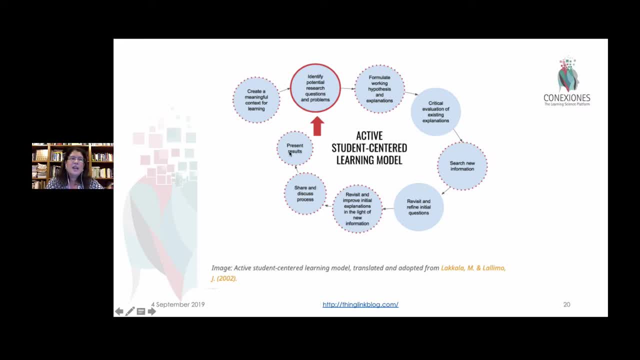 interaction in our class And we're going to see if that fixes anything. And the likelihood is, because of the great nature of teaching, it just goes on. Now we'll have a new kind of a question, a new kind of a problem, and this will continually be cyclical. okay, 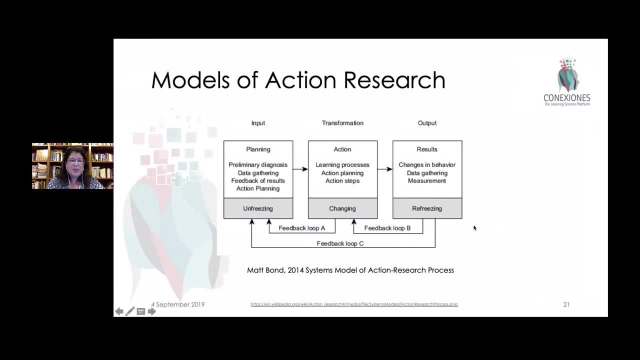 Another model. as Bond puts it, it's pretty much: you have a plan, You put that plan into action. Even the act of putting it into action might make you change your plan, But then you're going to get some results from that intervention you did with a kid, right, I plan to read out loud to the kids. 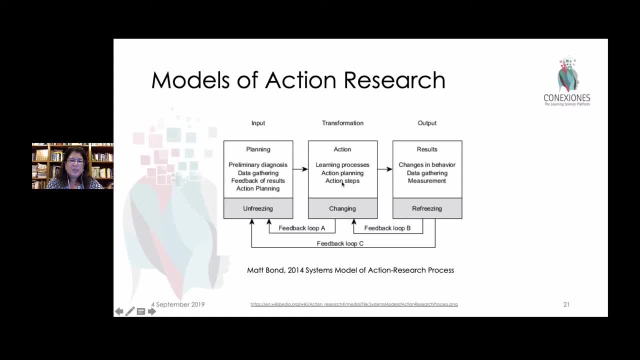 for 20 minutes a day. You put that into action, but then you realize that maybe it's better if they read to themselves instead of you read to them, And so maybe you're changing your ideas here. Then you get some results. Oh, it does seem like they're reading more for pleasure. 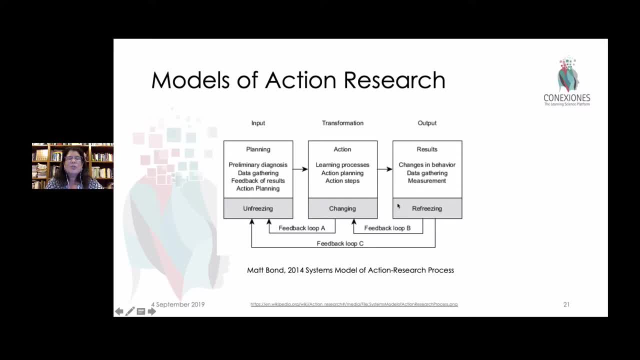 But then you have to rethink this And this is a general, again cyclical, process, even though Bond chose to make it with little squares, And I put his in here, his model in here. There's thousands of them, But I put his because it's one of the few that doesn't try to go in a 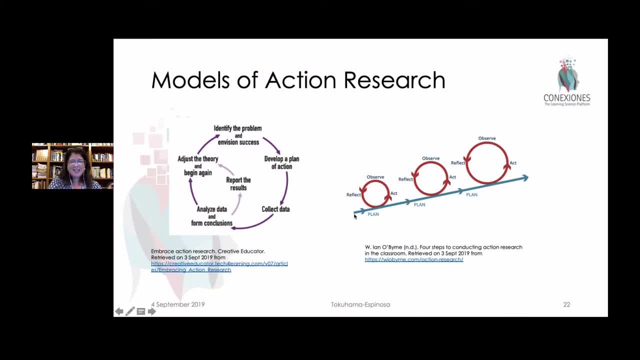 circle, Because most of the models will basically say: you know you have a plan, Let's put our plan into action. Let's observe what happens, Let's think about what happened, Let's reflect on that And then let's have a new plan And let's put that into action And then see what happens. Let's 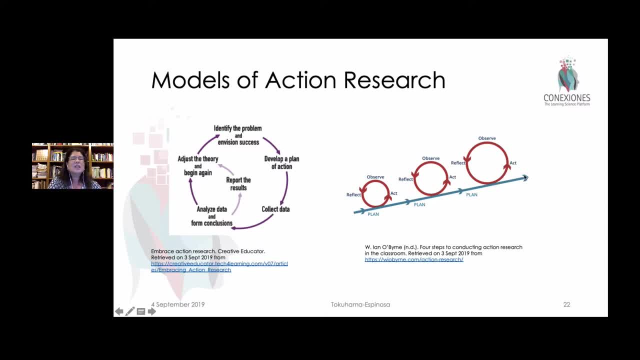 observe, Let's reflect on that, And then we have a new plan. So this is cyclical. The idea of action research is that this is an incredibly ongoing iterative process that never has an end, because each of our problems just becomes different and more. 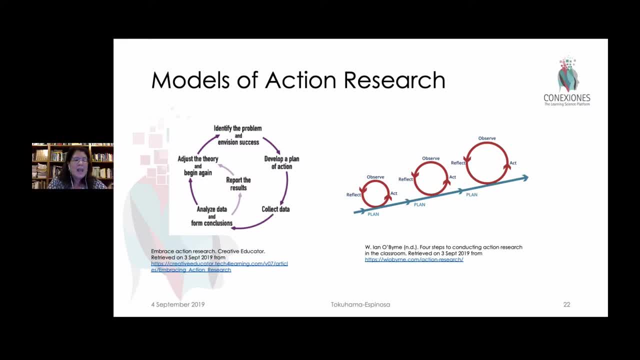 sophisticated, And that's the art of teaching, basically right. Others, you know, identify the problem, They develop their plan, They collect the data, They analyze, They report these things And then they adjust And then they begin again. So this describes the same cyclical process. 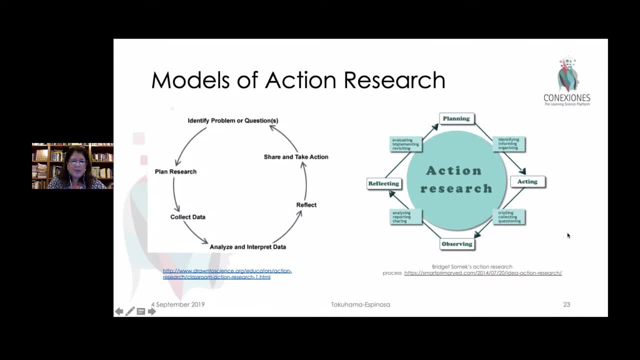 but sort of in an ongoing way. here, Other models are very, very similar. The biggest difference here is that the arrows go in the different directions. So you identify a problem, You plan the research, You collect the data, You analyze, You reflect, You share this. 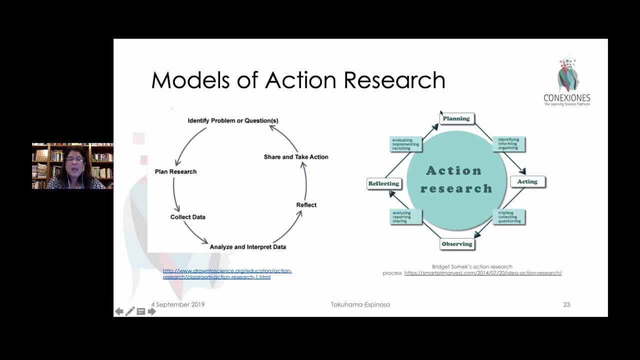 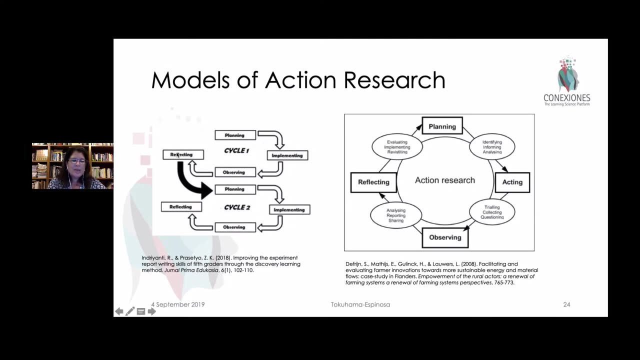 You take action And then you have a new problem. That's the way it goes, right. But these four key stages of planning, acting, observing and reflecting are basically the classic steps of action, research, right. So we plan, We implement or act. We observe what happens, We reflect on. 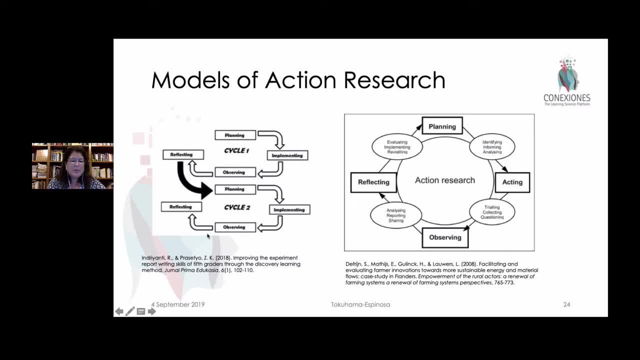 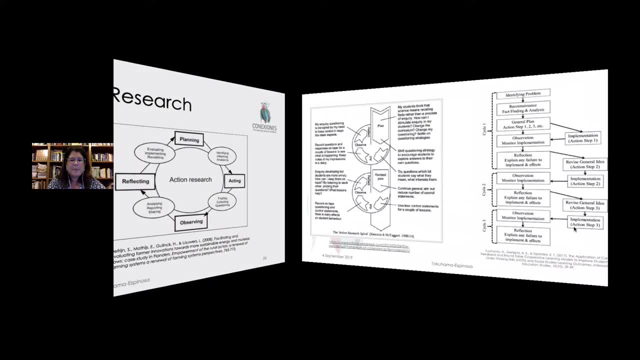 this And then we start again. We plan, We implement, We observe, We reflect. right, Plan, act, observe, reflect. All of this is basically an ongoing process, right? Probably one of the most seminal articles ever written on. 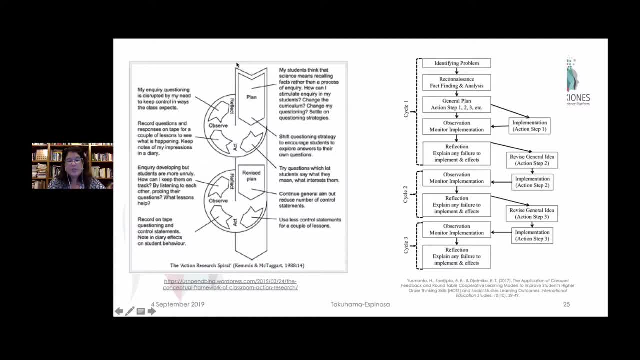 this was done by Chemist and McTaggart in 88. Here's a concrete explanation here of you know this is my plan. This is the background information I had. This is the action I put into place. I observed what happened with the kids I think about. you know how they reacted to that particular. 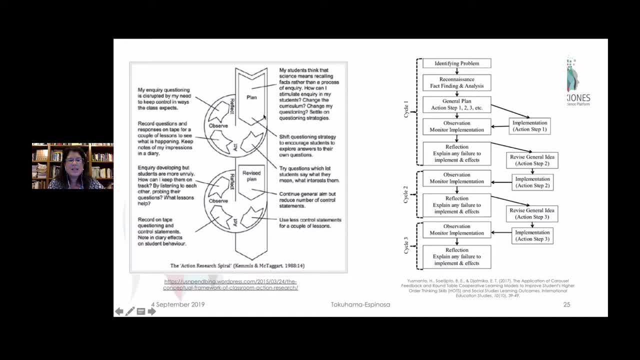 teaching, And then I've revised my plan and now I have a new one. So his is kind of a little bit of a bit different, but it was one of the first to get out there right. Same thing here: Identify problems, Reconnaissance, fact-finding and analysis. This is basically what we're calling. 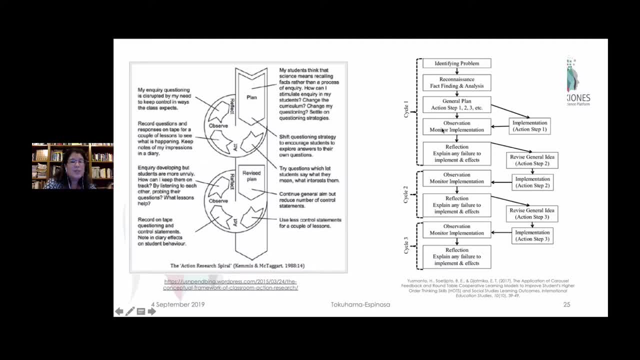 the literature review, You make a plan about what you're going to do, You implement it and observe what happens here, and then you think about what happened there, And all along the way we have basically adjustments to our own teaching practice based on the results that we have at each of these. 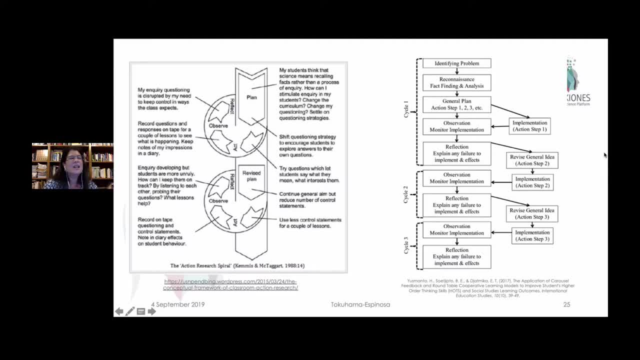 different stages, And that's the real beauty of teaching- is that we do this every single day For 20, 30 kids in our class, over and over, and they're almost unique to the individual kid. We'll have a global plan, but some of the kids we're going to need to adjust this and do things slightly. 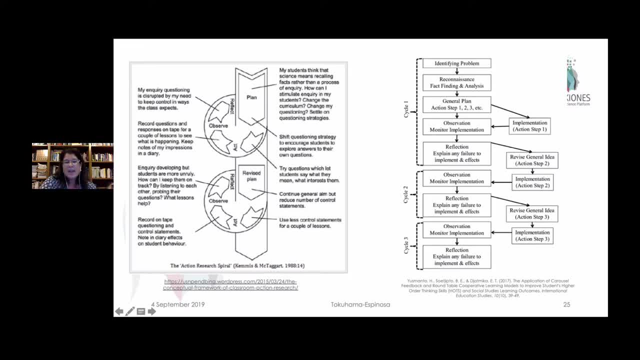 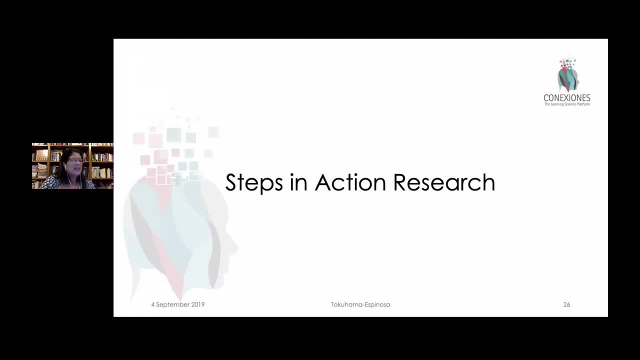 differently, based on the entire dynamics of the class. And that is part of the beauty of teaching and one of the reasons it's so hard to document our practice. So last part: here let's look at seven steps in action research. Now there were multiple steps. We said that there were those. 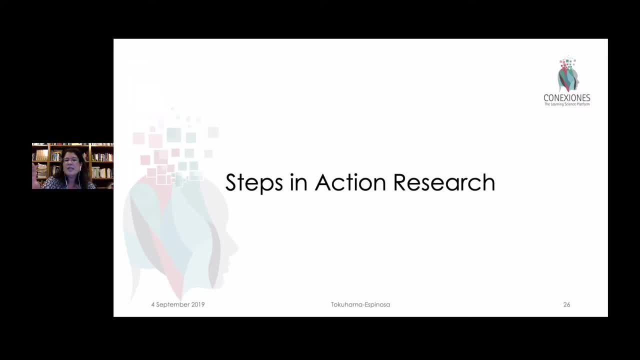 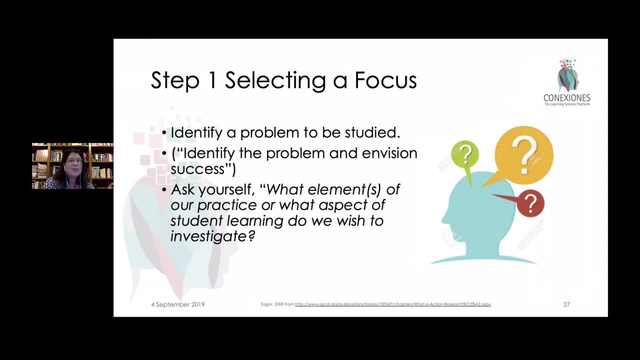 four core ones there. Let's just look at this as seven steps to follow, And then we're going to make sure that we've created a great action research project. The very first thing we asked you to do when we met you was to come up with a problem or identify things. What do you want to? 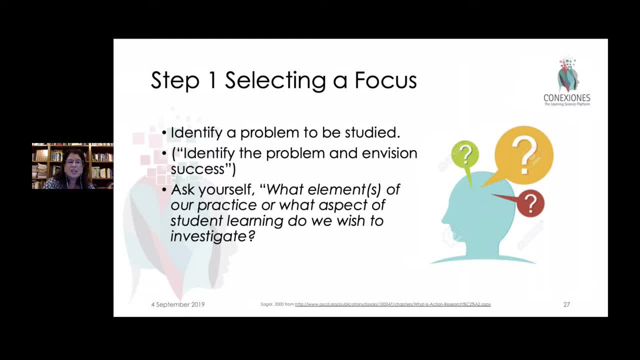 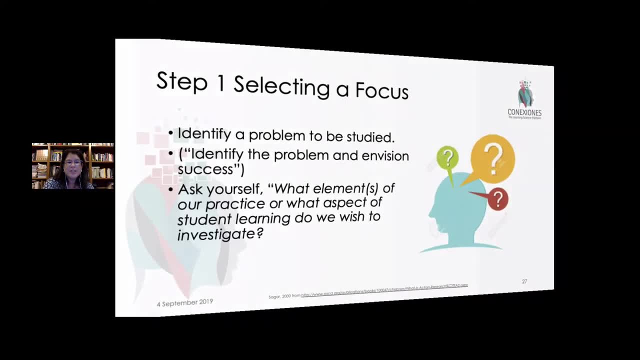 know right And identify something that you would like to conduct your action research on. So what is it that you would like to improve or understand a little bit better, to be able to be a better teacher? The second step we had in our process was to connect what you wanted to know to a research. 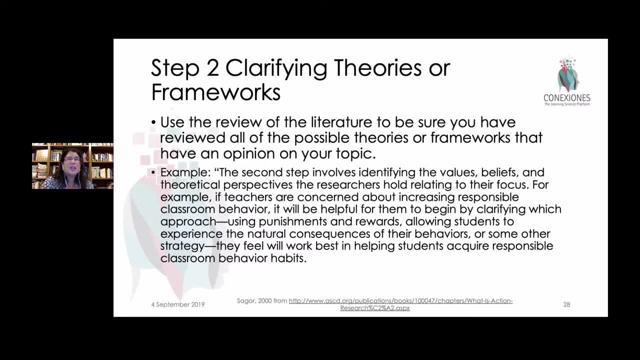 question. In this sense, we've incorporated here this onion level, which was basically saying: also think about your philosophical approach to this whole thing. What theoretical frameworks are you using to approach this? This is important mainly because we want you to have a balance of thinking So, as you were doing your literature reviews, we really wanted 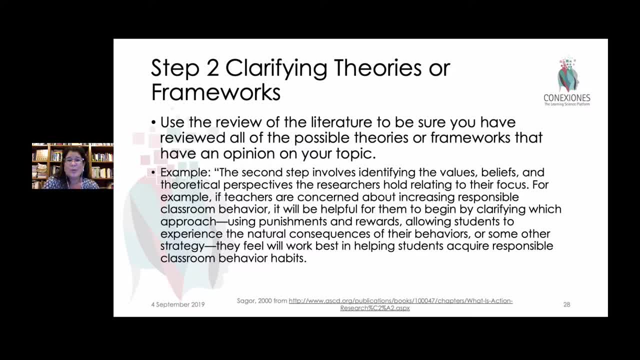 to push you to think about finding things that maybe disagree with what you think is true, Mainly because these different theoretical frameworks, the different approaches, will expand the way that you can now understand that problem right, And so this is a very important step. 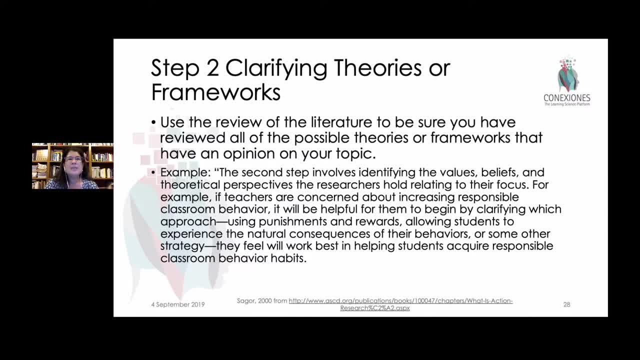 It's one that takes a lot more time and that often times, in action research, design in teaching and classroom settings, we don't spend enough time doing it, But we throw this in as another step that we hope that you're able to take, though we are not doing it actively within this classroom structure. okay. 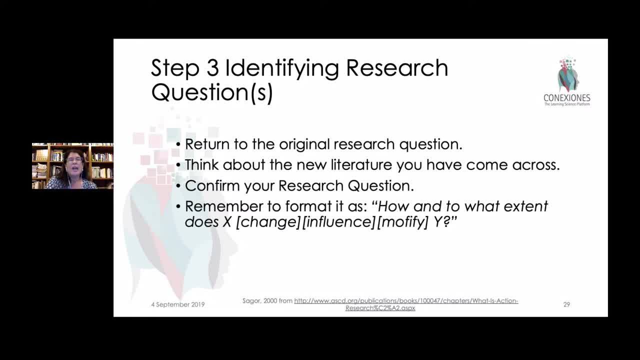 So then you come up with your research question and after you've reviewed the literature, we want you to revisit that question. okay, Think about how your question might be changed by some of the new things that you've learned through the literature. And to rethink that research question. has your question changed Now? has it been modified by the new information that you now have? 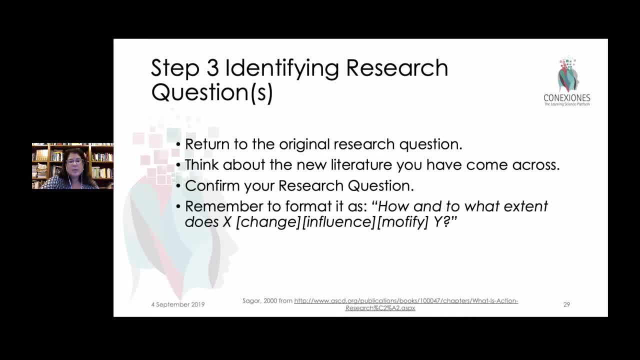 And again reframe it in that structure, If possible. you know how and to what extent does X influence or change Y, Because isolating those variables gets more and more important the more information we have. Classroom settings are incredibly messy and the reason that research is so difficult to conduct is that it's very, very difficult to pinpoint. 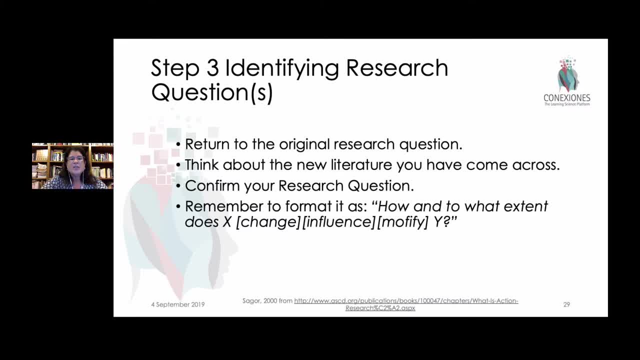 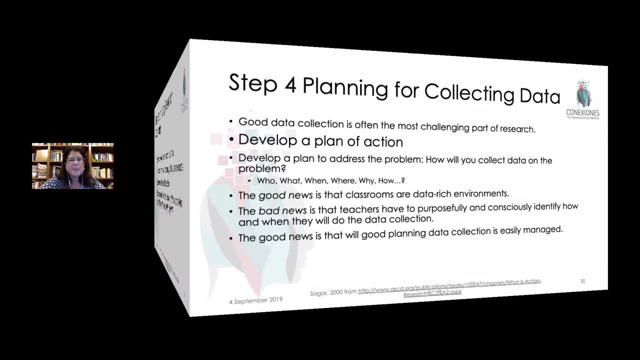 what is actually influencing what else. So, in order to do this clearly and cleanly, we really want to force you into this research structure, if possible, this questioning structure. The fourth step has a couple of different stages. The main idea here is that, before you collect your data, before you. 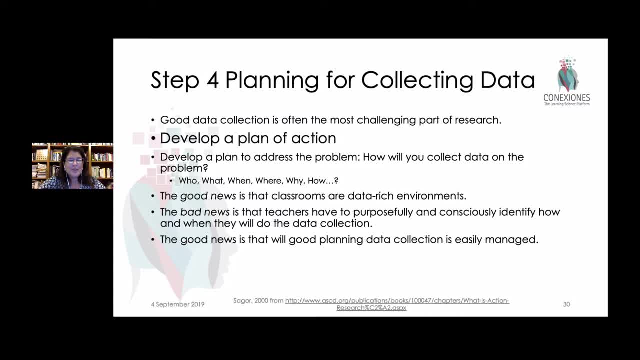 launch out there and just apply the tool. think about your plan. What is it you're going to do? How are you going to approach this? Who is going to be involved? What's the timing of it? The main idea is that the data collection process of this stage is pretty much the most complicated. 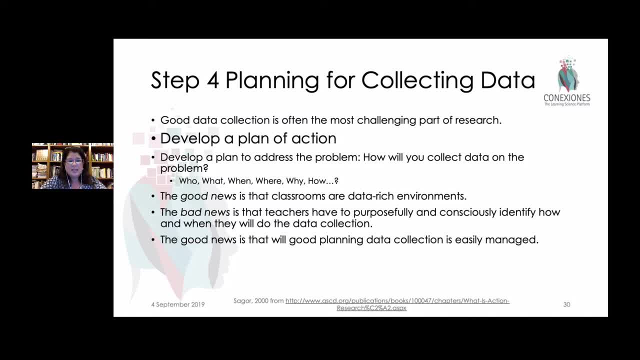 But if you have a gut Middle East experiment and then you want to approach this, you want to need good plan, it works out really easily. So this is the big idea is: let's take a step, let's think about this. I'm going to do a pre-test and I'm going to do a post-test, and that's going to be. 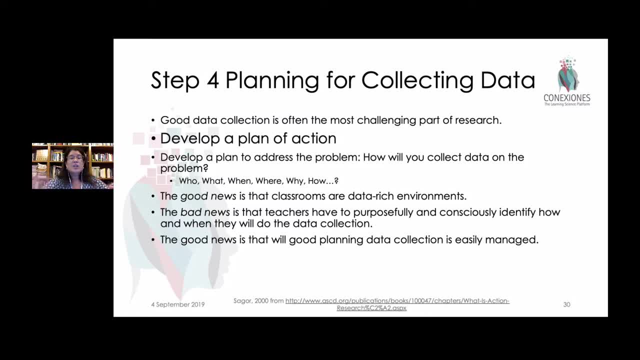 my data gathering, Or I'm going to collect journal entries digitally throughout the semester and then I'm going to compare the growth in their writing as far as number of words or new vocabulary, whatever it is. Make a plan about how you're going to do it and when you're going to do it. 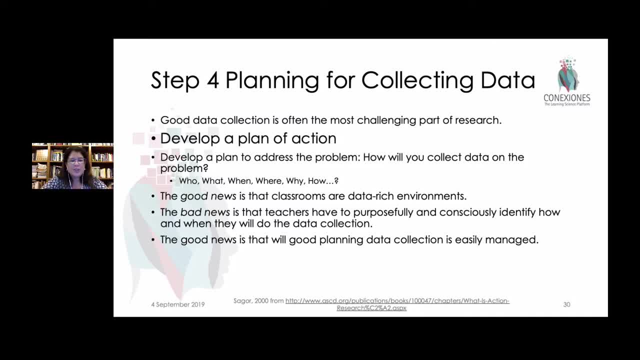 and that will save you a lot of problems in the long run. The good news is that classrooms are data-rich environments. The bad news is that we really have to take this time to purposely and conscientiously identify how we are going to be collecting that data. But the good news again is: 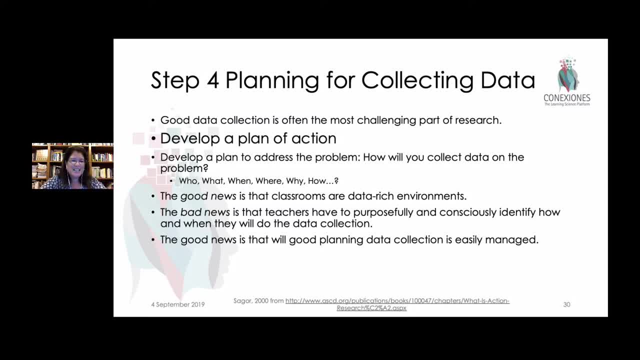 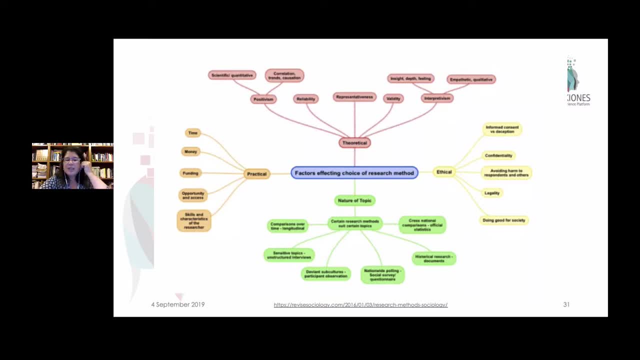 that once you've got that plan, it's really easy to follow. So hopefully we'll take the time to do that planning when we're together in class, okay. Another thing to take into consideration is sort of looking at that research onion model, but looking at it as more graphic form. here is take. 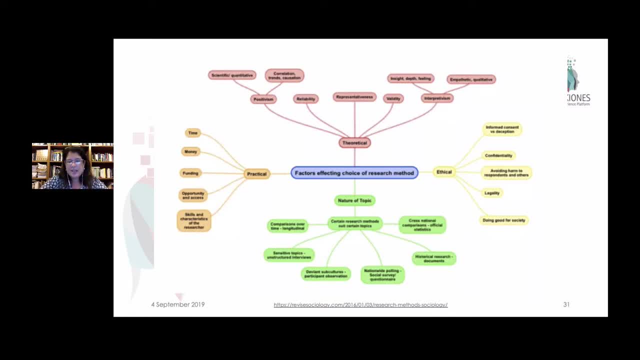 into consideration as you create that plan, other things that you're going to be collecting, So the theoretical frameworks that you have in mind, ethical considerations, what your topic is, the nature of your topic and how that might lend itself to a specific tool. But, more than anything, 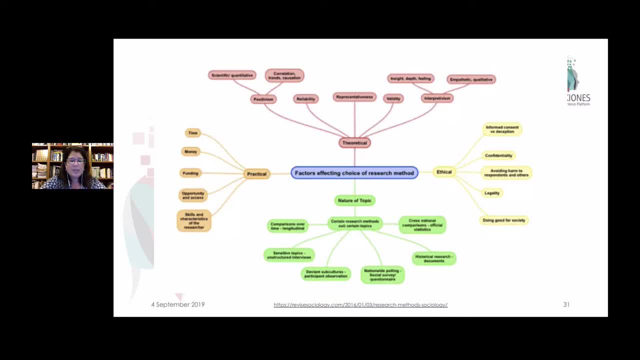 be very practical in the sense of how much time you actually have to gather that data, if you have access to those data sources that you're looking for, if you're depending on other people to be able to collect that data or not. So make sure that those things are all taken. 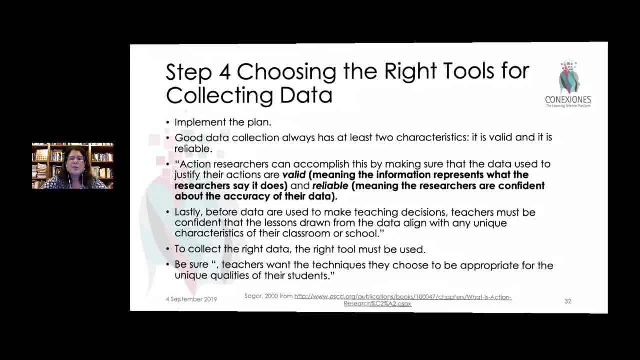 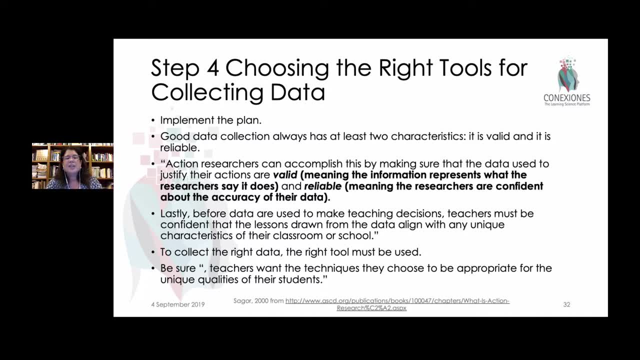 into consideration as you choose your tools. So, once you've chosen the methodology, once you're clear on the data tools that you're going to be using and you've implemented the plan, make sure that you're thinking about the data collection, at least on two different levels. 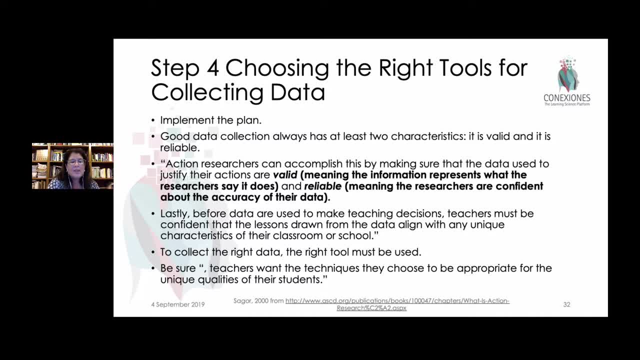 All great data collection has at least two things in common. First, the data is valid. That means that the information that you think is represented by what you've collected is so right And that it's reliable meaning: the researchers are confident about the accuracy of their data. 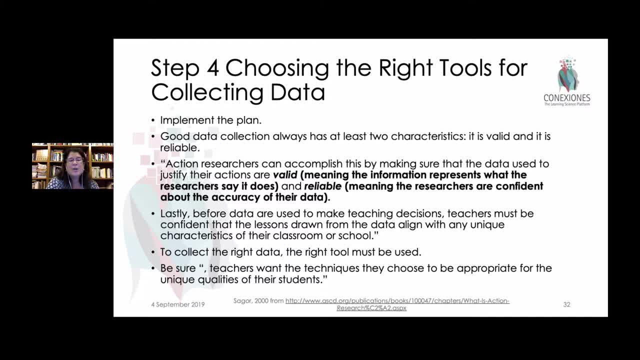 meaning it can be replicated by other researchers. So validity, for example, is a very important aspect of data collection. So, for example, you might have a huge mistake when a researcher might presume that they have shown that mathematical reasoning in students has 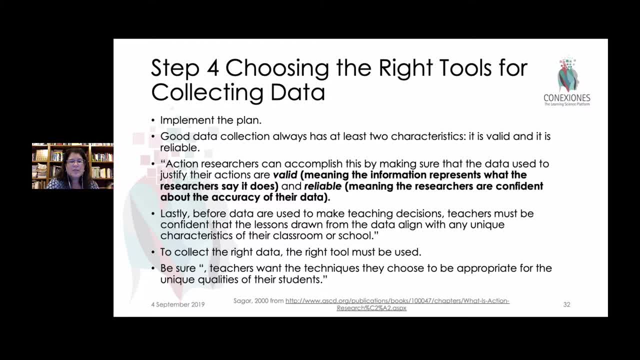 increased because test scores on a specific test increased. Well, that's not exactly true. There's a lot of interpretation there, right? Or you might presume that, since you increased total number of school days from 180 a year to 200, that students are learning more. Well, the truth of the matter. 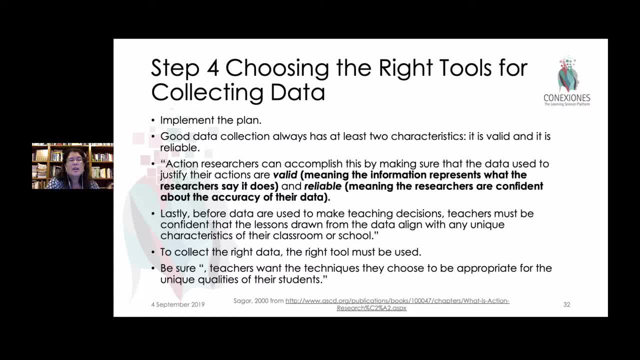 they're just going to school more. It doesn't mean that they're learning more, right? So one type of data to come to conclusions that don't bear the weight of that data. okay, And in terms of reliability, this basically means that anybody could take your research protocol and if they 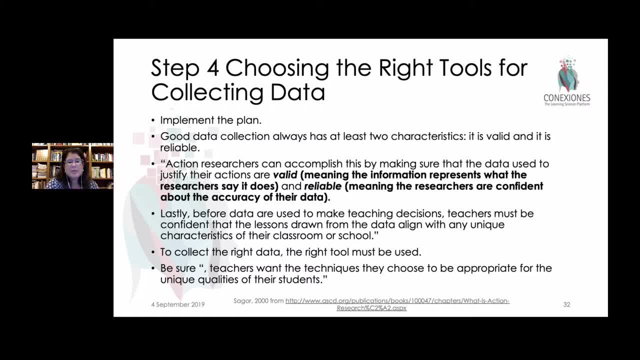 followed it, they'd get the same results. So the idea of reliability means that what you are putting forth is something that could be replicated by other researchers. okay, So all of this hinges on the right tool, Choosing the right tool to measure and to gather the data that will give us the 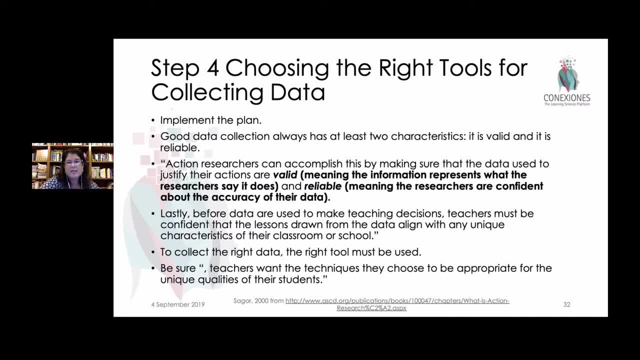 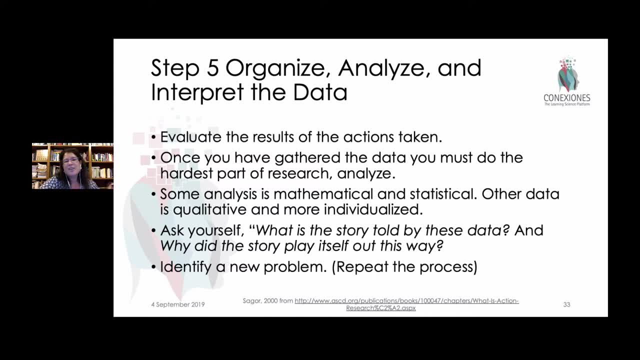 evidence that we are able to respond to the research question that we've planted in the first place. The fifth step, then: once we've gathered all that data, what we have to do is now take that big collection of information and organize it, analyze it, interpret it, And this is probably 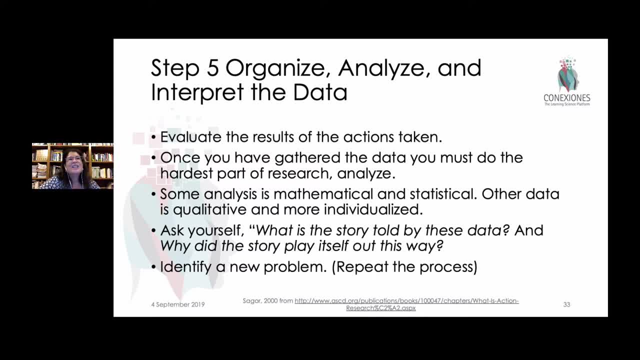 the greatest stage of research, because it's the point where you stop reporting what you found from other people. and now this is really a lot higher order thinking. And it's one thing to report children's test scores appeared to go up and students reported that. And it's one thing to report children's test scores appeared to go up and. 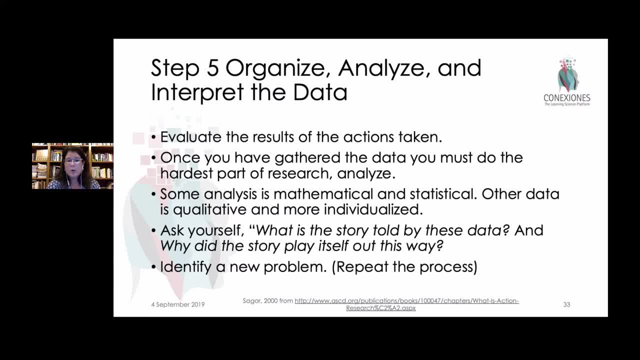 students reported that, And it's one thing to report. children's test scores appeared to go up and students reported they liked the intervention. Well, that's reporting and that's nice and that's good information, But the why their test scores went up and why did they enjoy that particular. 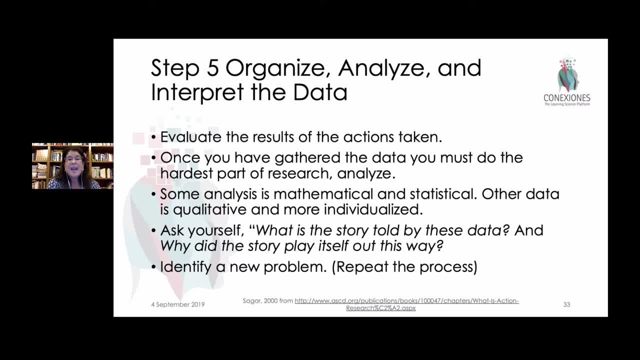 type of teaching activity or learning activity more. that is higher order thinking. So remember to go back to Bloom and Bloom's taxonomy and remember these different levels here. Reporting, just understanding, is a very base level, right, But to get to this level where 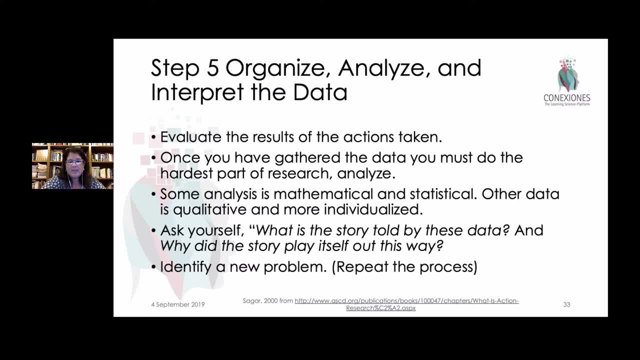 you can analyze and interpret and explain the why behind the findings is a very important thing, And that's really the beauty of most of the research is to get to that why. That also means taking not only the data that you've gathered but combining that with a review of the literature. 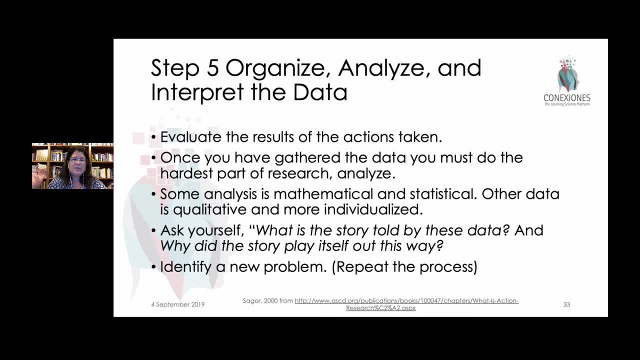 that you did beforehand and looking what past people have also found in similar contexts. Combine that with your own data and now what is your vision on your problem? So the key idea here is: once you've resolved or identified or analyzed the information, now you can actually grow that. 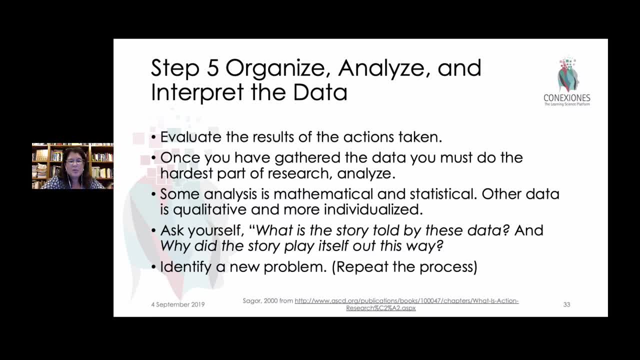 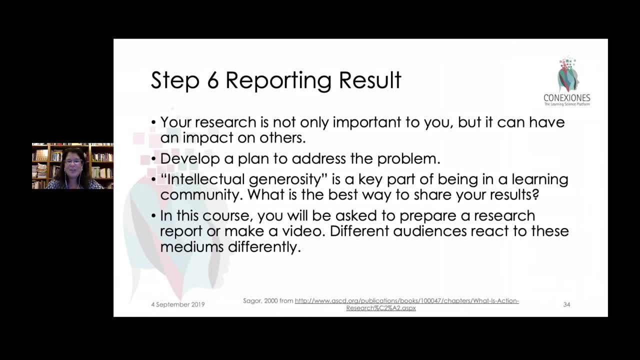 problem, And that's really the beauty of the research, And that's really the beauty of the research. So the penultimate step is reporting your results. So, once you've got all this great information, you've got the whys behind all this information. it's not only important to you, It's 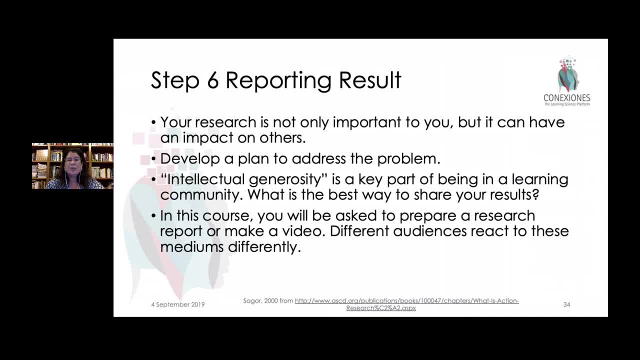 great that you know the information, but sharing it with others is huge. So come up with a plan about how you're going to be sharing these results and how you're going to be intellectually generous, how you may be saving somebody else from similar problems in the future, because you can. 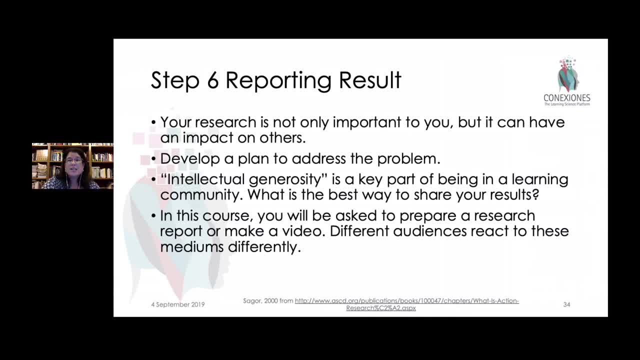 explain to them within the data that you've gathered, And that's really the key thing Within maybe the Kamehameha context seems to be true for 10th and 11th graders. This is what I found with my data. Hope you can try to replicate it as well. It'd be great because it may change certain. 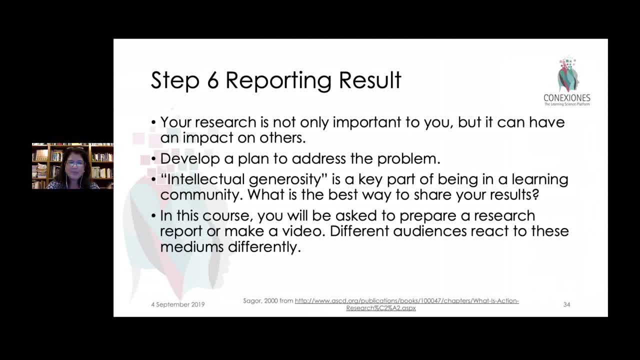 policies about the way we interact with our kids, for example. Okay, So you're asked in this course to prepare a way to share your results. It can either be a video recording or it can be a paper, but what we want to do is to share and give back to the community, because this is another step in 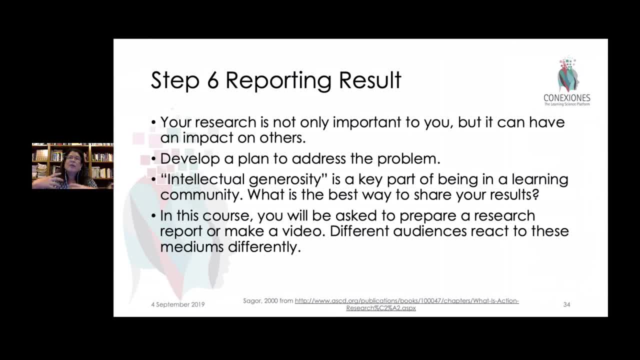 your own thinking process. You have to be able to share your results. You have to be able to share your results. So we've got a specific way to share your data, for you to be able to share your results. So you're going to have an idea. You had a problem. You're going to take the time to do research on it. 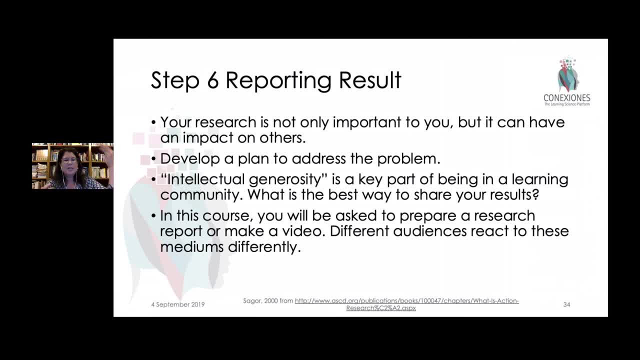 You're going to do an intervention, You're going to have data And you're going to come to now a new understanding of that particular problem, And once you put that out to the world, it again will change people's feedback the way they see it. They might find other types of whys or analysis. 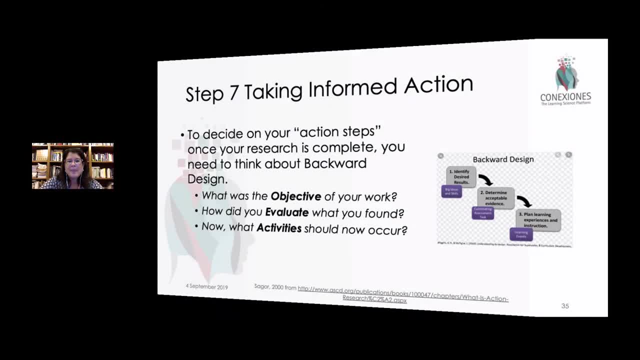 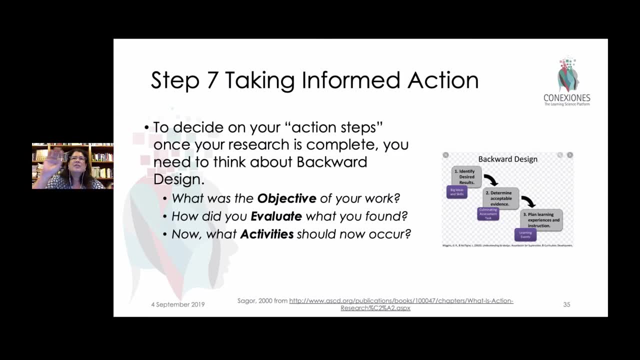 that maybe you didn't see. This will add to your growing understanding of your particular topic, and the last step is to take action. Now that we've had that entire feedback loop, now that we've had this problem, this intervention, we have our findings, we understand the information better. 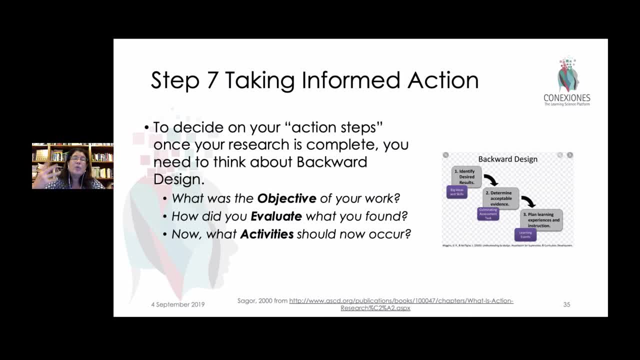 we've shared it with the outside world. we have a new vision now. now, what do we do? This is basically backward design thinking. right Go back to the original objective of your work. What was it that you wanted to know? Now look at the tools that you used to gather data, and how did you? 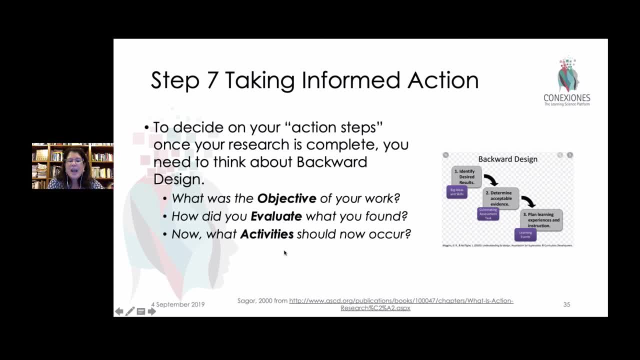 evaluate and answer your research question. And now, now that you have all of this information, where does that take you? How do you do something different or new within your own class structure? Do you want to recommend a different kind of a policy? Will you just change your interaction? 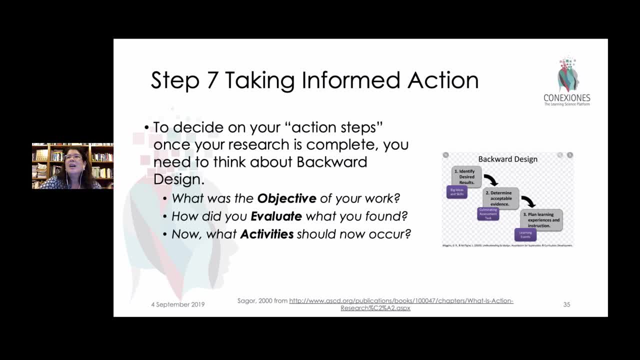 with the students. Do you want to recommend that everybody teaches science by going out to the fish pond? I don't know. there's maybe a hundred different things that will come out of this, but the idea is to now take action. The key idea of action research is that 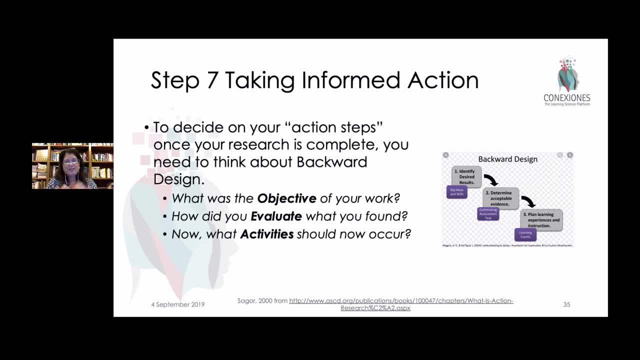 you act upon information that you have interpreted, and now you're going to do something even better the next time. That's a beautiful scientific background. in this art of teaching, We continually do action research on a daily basis in our heads. The big idea is: